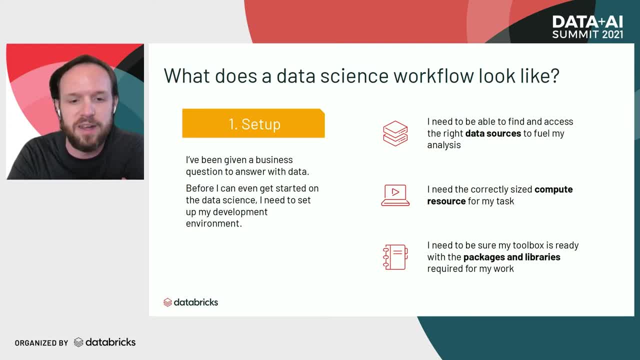 and access the right data to do my analysis. I need to get a correctly sized piece of compute for my task And I need to get my toolbox ready with the packages and libraries I'll need for my work. But that's just the beginning. Once the overhead of setup is complete, the 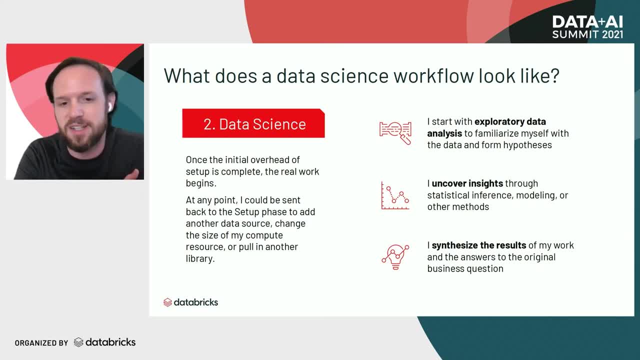 real work is going to begin. I start by exploring the data I've collected so that I can make sure that I can familiarize myself with it and form some hypotheses, And then, using methods like statistical inference, visualization, modeling, I'll uncover insights about the 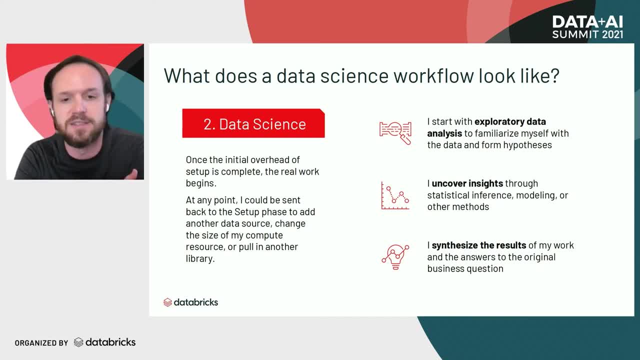 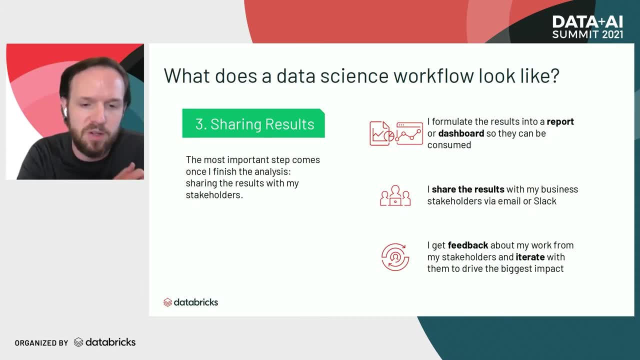 data, And then I'll finish the analysis by synthesizing those insults and results into answers to the business question that started the project. The most important step in the whole process comes next: sharing my results with my stakeholders so that all my work, all that time I spend, has an impact on the business. To do this, 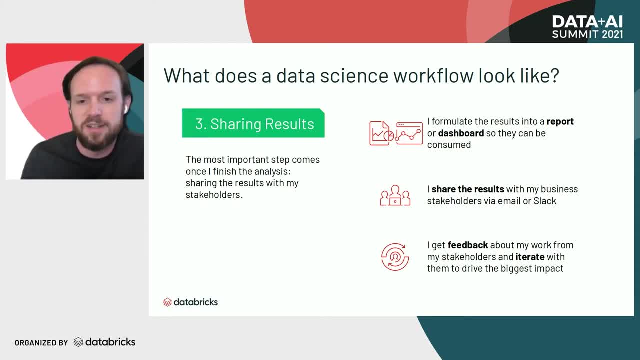 I'm going to package my work into a data science project. I'm going to start with a data science project. I'm going to put my work into a report or a dashboard that my stakeholders can easily consume And I'll share it with them via email or Slack or some other channel. 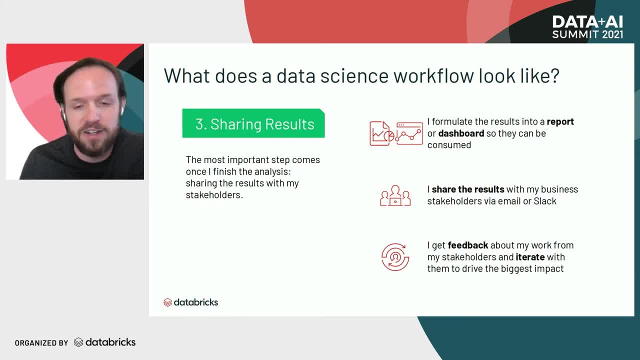 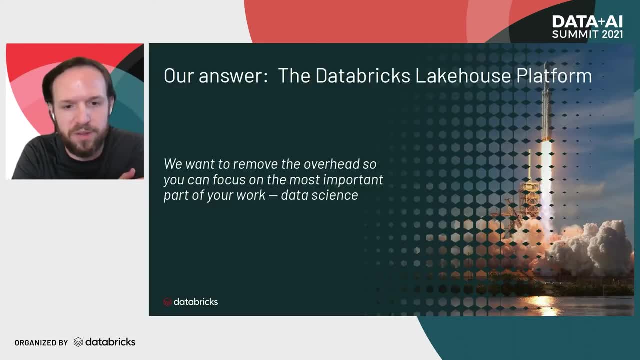 From there, I gather feedback about the work and iterate on it with those stakeholders to drive the biggest impact I can. So how does Databricks work with you through this workflow? Our answer is the Databricks Lakehouse platform: a unified place for all. 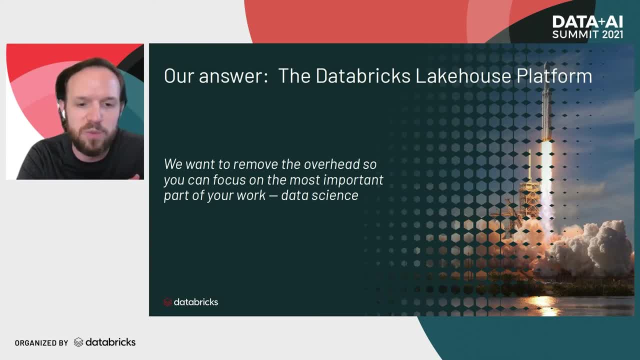 your data and data analysis. With it, we want to remove all this overhead of setup and configuration so that you can focus on the most important part of your work: the data science. The Databricks Lakehouse platform is unique in three ways. It's simple: All your data. 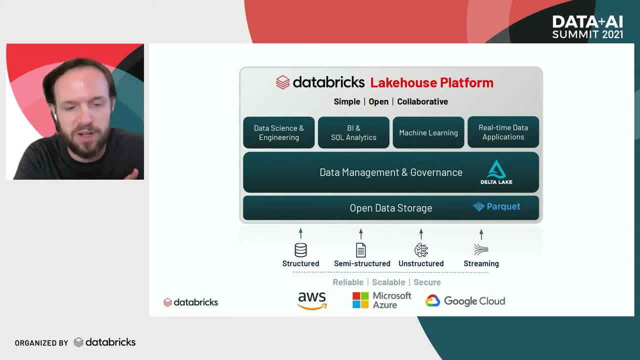 comes together in one place so that all data workloads happen on one common platform. It's open. It's based on open source and open standards to make it easy to work with existing tools and avoid proprietary formats. Finally, it's collaborative: You can work with other data scientists as well as data 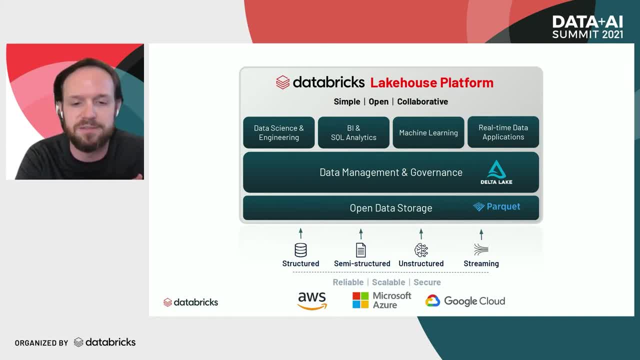 engineers and analysts to deliver your vision and to improve the job searchleist. Кин protocol analysts to deliver insights that have an outsized effect on your business. Putting this all together, this is why Databricks is the data and AI company. No one else can do what we can do with a simple, single solution. 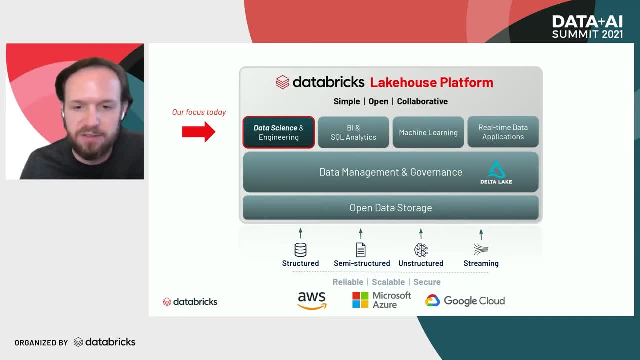 So in this session, like I said, we're just focusing on the data science part of the lake house. Please check out other sessions for deep dives into other parts of the platform. So how does Databricks work with you when doing data science? 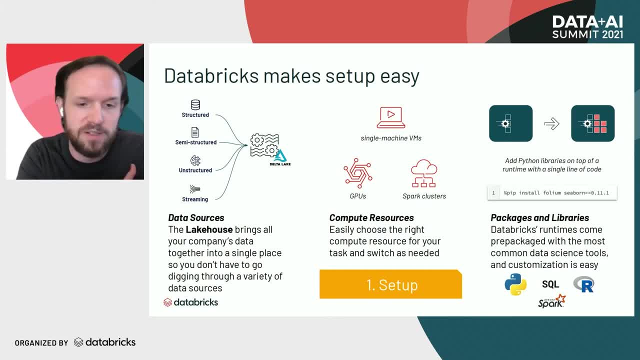 First off, Databricks makes setup easy. All your data sources are in a single place. The lake house brings them all together, so you don't have to go digging. You can then easily choose the right compute resource for your task, And that can be anything from a single machine VM to a VM with a bunch of GPUs or 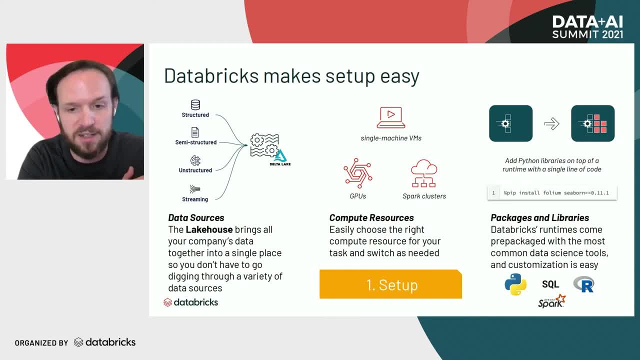 a big Spark cluster And you can switch between them as needed. Finally, Databricks comes with a single machine VM and a big Spark cluster. Finally, Databricks comes with a single machine VM and a big Spark cluster. It comes with runtimes that package together all the standard open source data science tools. 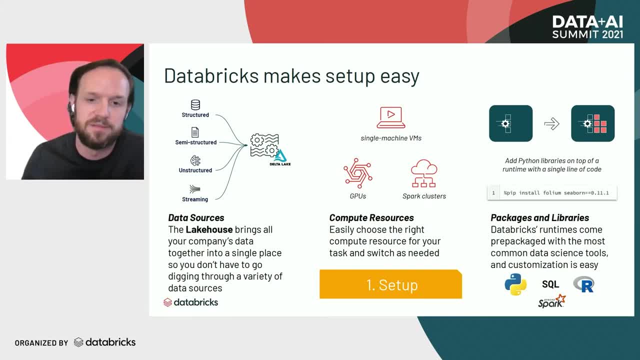 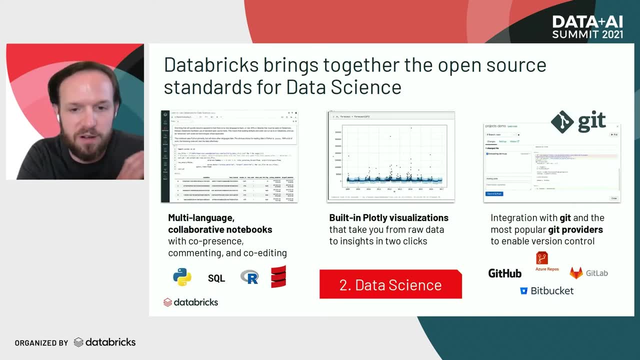 And it's easy to customize your environment to add new ones. Continuing on the theme of open source tools, Databricks brings together all the open source standards for data science development. The Databricks notebook supports multiple languages, from Python to SQL or Scala. 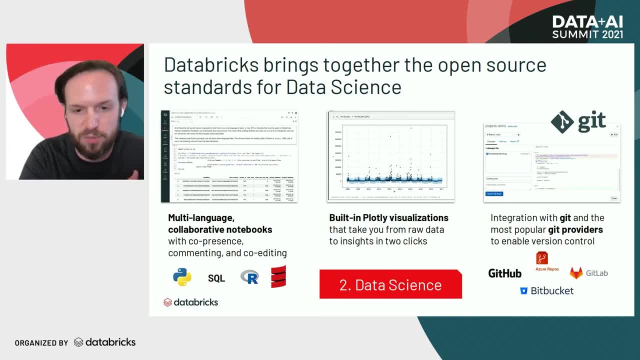 And it enables you to work with your colleagues in real time with co-presence in our notebooks, commenting in our notebooks and co-editing. The notebook also comes with built-in plot lead visualizations, which you can use to quickly derive insights from your data with just two clicks. 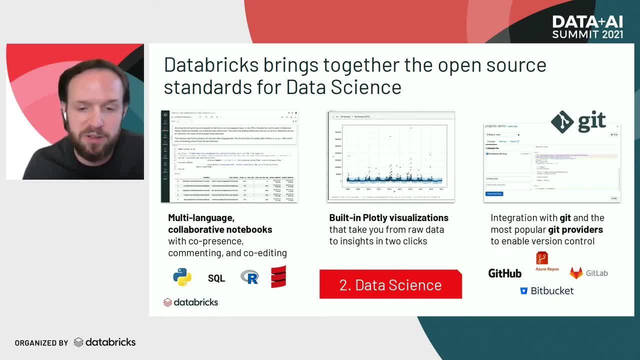 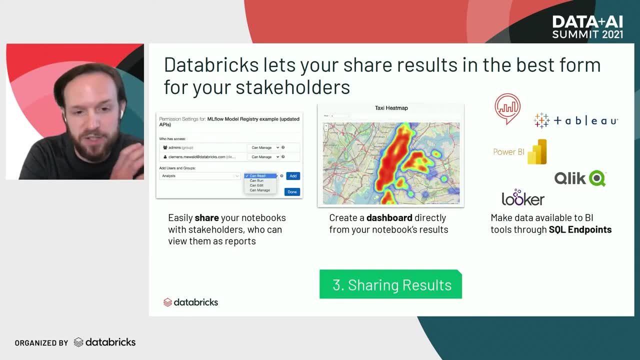 Finally, the notebook is also integrated with Git and the most popular Git providers to support finer-grained version control. Lastly, when you're finally finished with your analysis and all that hard work, Databricks helps you to share your results in the best form for your stakeholders. 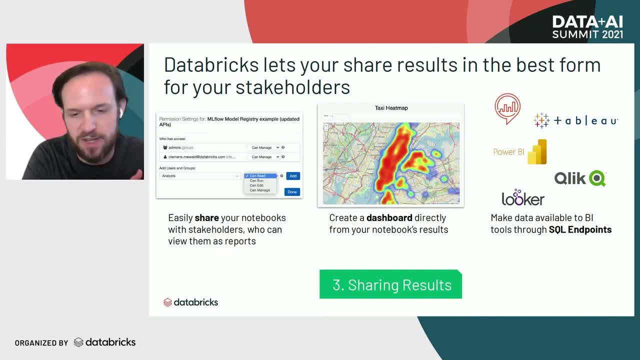 You can easily share your notebooks as reports, just by giving those stakeholders access. You can also quickly create a dashboard to share your results with your stakeholders. You can also create a dashboard directly from the outputs of your work in the notebook. Lastly, you can make that data that you process any new data you may have created. 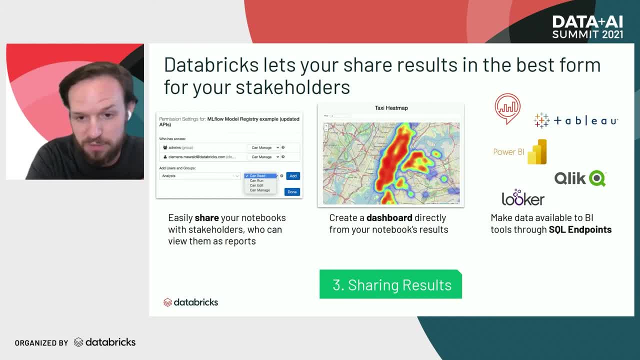 available to BI tools like our own SQL Analytics, Tableau, Power BI and others through Databricks, SQL Endpoints. Now to get practical and show you how it's all done, I'm going to turn it over to my colleague. 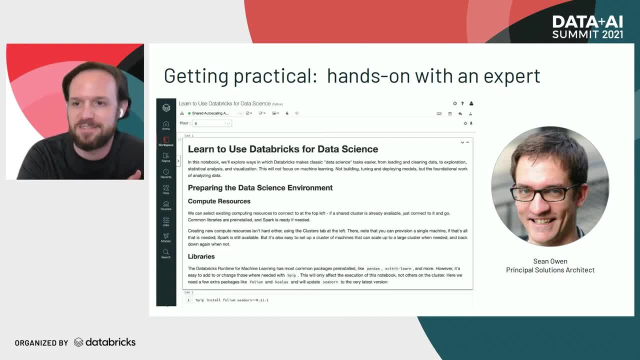 Sean, who's going to walk you through a hands-on demo. Take it away, Sean. Great Thanks, Austin. Hello, Welcome everyone to the Spritecom webinar. I'm going to talk to you today about how you can use the database to create your own SQL analytics. 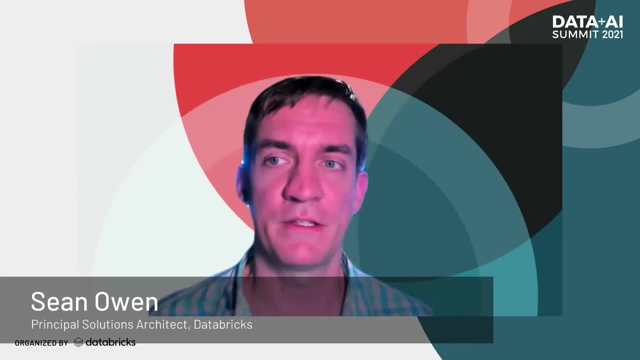 I'm going to turn it over to my colleague, Sean, who's going to walk you through a hands-on demo. Take it away, Sean. Great Thanks, Austin. Hello Welcome everyone to the Spritecom webinar. Great Thanks, Austin. Hello Welcome everyone to the Spritecom webinar. 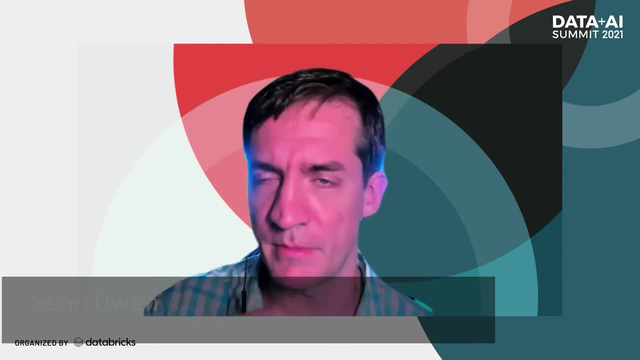 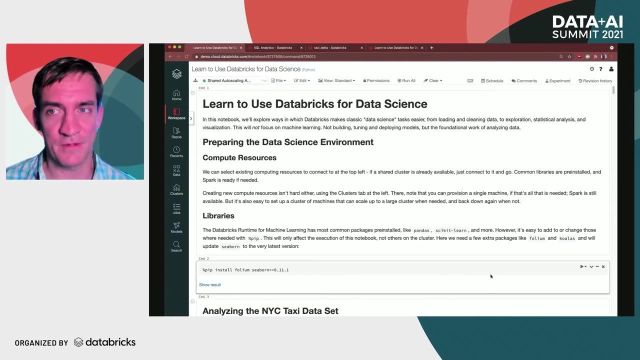 And, as Austin alluded to, I'd love to show you how to do data science on Databricks. So, as Austin alluded to, we're not going to do machine learning here. We're not going to use MLflow here. We have other sessions for that. We're not going to do data engineering either. 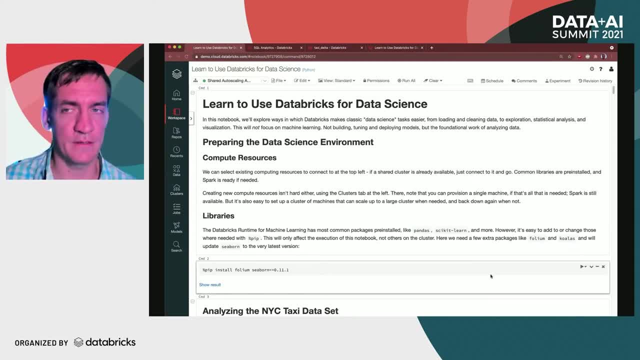 This session is directed at people who maybe are working in Python or R to analyze data, get insights from data, maybe fit statistical models to data as well. traditional data science. I want to show you you can do these things on Databricks in the same way you do it anywhere. 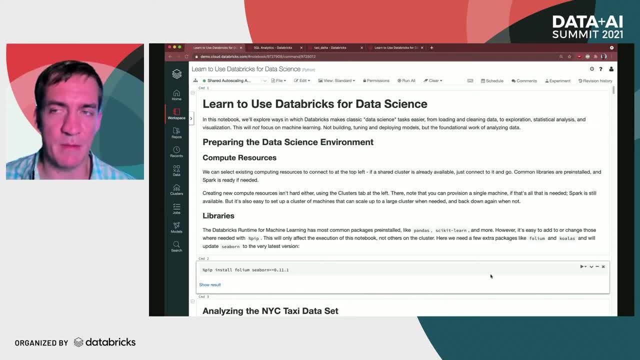 else, but we provide some enhancements to make your life easier or help you scale up to larger datasets. First of all, for those that are new to Databricks, this is Databricks: what you'll be looking at, the environment you'll be using if you use. 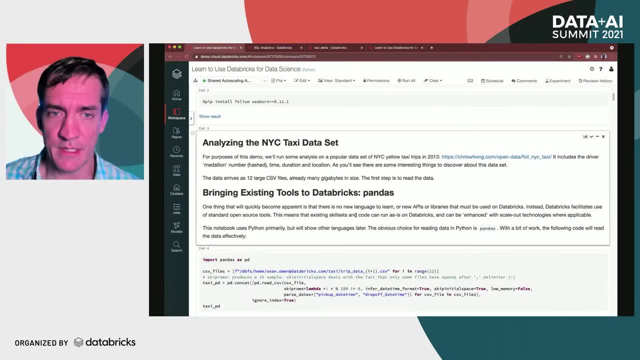 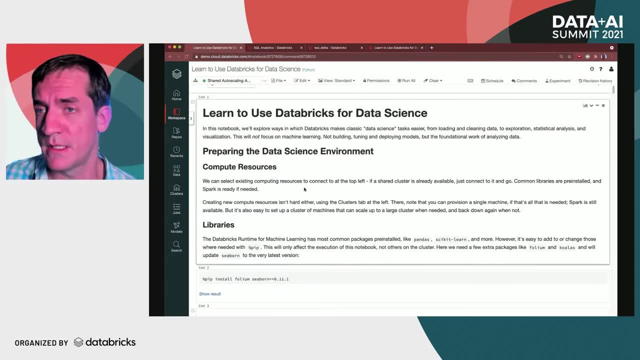 Databricks. It's a notebook like environment where you can write code, execute code, see the results and, of course, write and mark down cells that document what you're doing- doing as well- And I like to tell people that there's really not much more to see in Databricks. 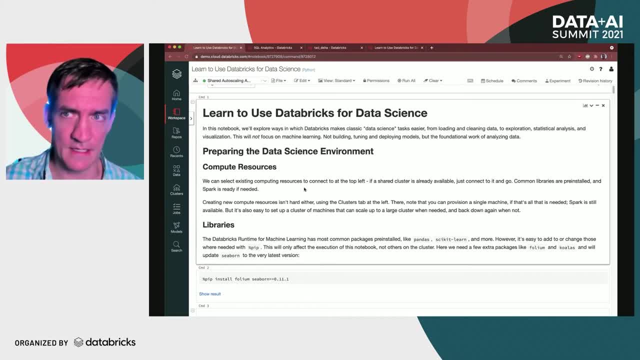 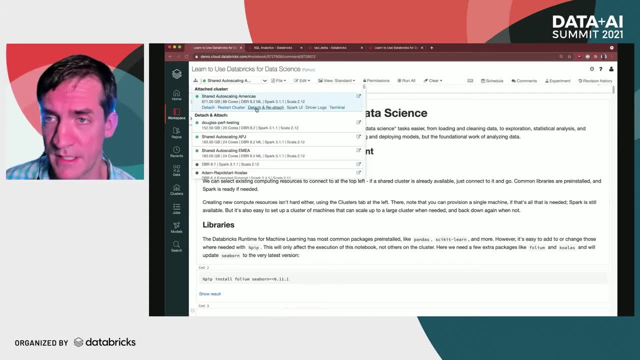 if you're a data scientist, You don't really have to deal with things like: where's my data, Where are my compute resources? In this case, I'm just going to connect to a shared Spark cluster here, Even though some of the stuff I'm doing is not going to be using Spark. you as well may be in. 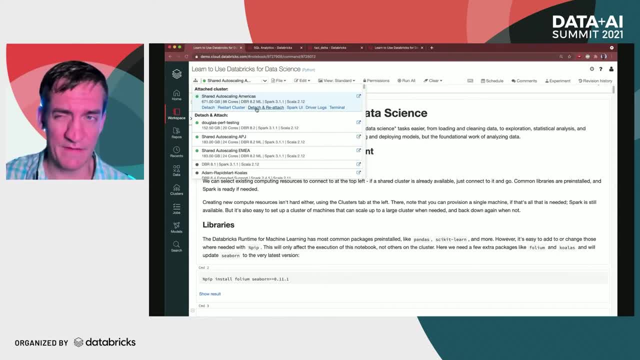 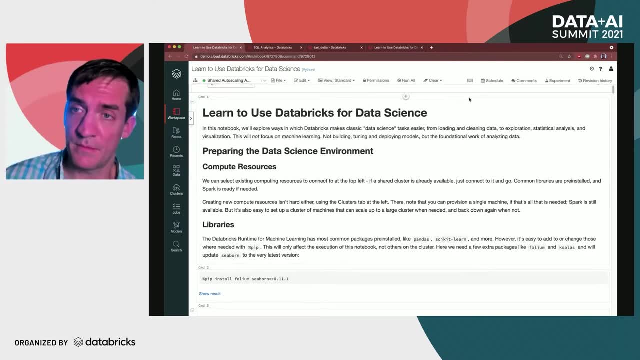 an environment where you just connect to an existing cluster. You don't even have to think about the compute resources in the cloud. They're there, They turn on. if they're not on, They turn off if they're not used. They scale up, They scale down. You just really don't have. 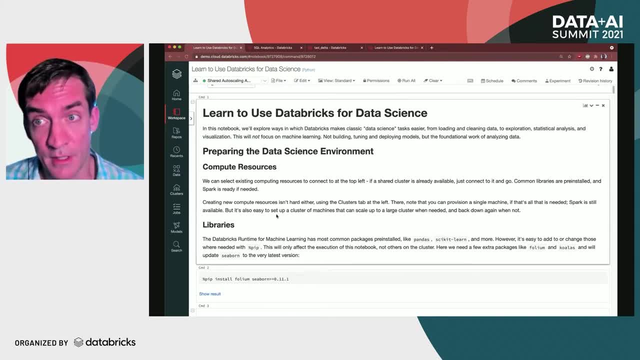 to think about it. And likewise for libraries. So you are probably using a lot of common libraries in Python or R. So in our runtime, in our ML runtime here, which I'm using here, most of the libraries you probably are using are already installed for you, whether it's in R. 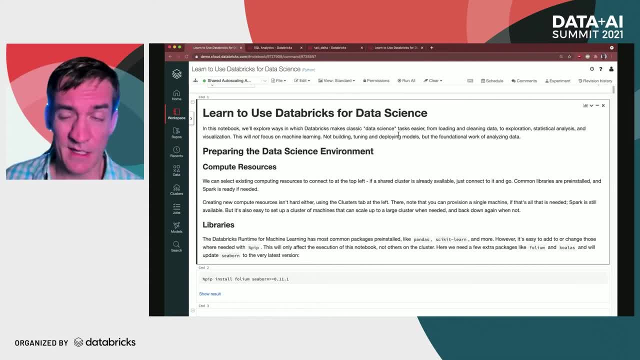 Python, Scala, et cetera. You don't have to worry about it In this case. I actually am later going to use a few of the libraries that I'm using. So I'm going to use a few of the libraries that I'm. 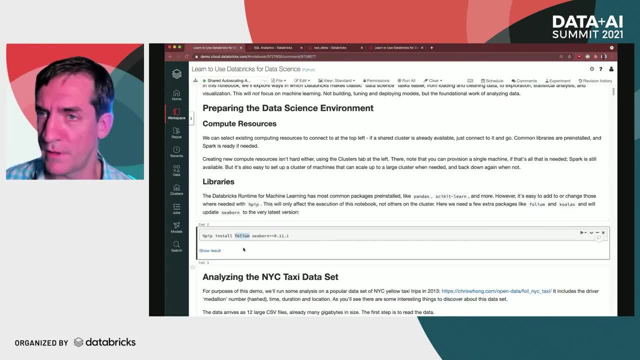 using. I'm going to use a few libraries that are not pre-installed in the runtime. One is called Folium, And I also want to update the version of Seaborn that I'm using. I want to use some really new features of a package called Seaborn, But the message here is that's really easy to do as well. 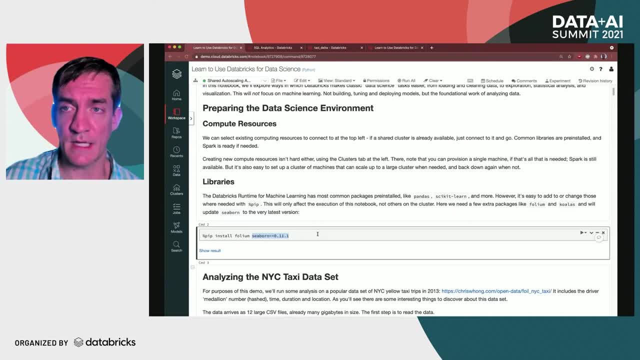 You can just pip install those libraries, those dependencies, and they only affect your notebook and your execution. So there's no worries that you're changing the environment for other users of some shared cluster. even if you're sharing a cluster, It's fine, This just affects your notebook. 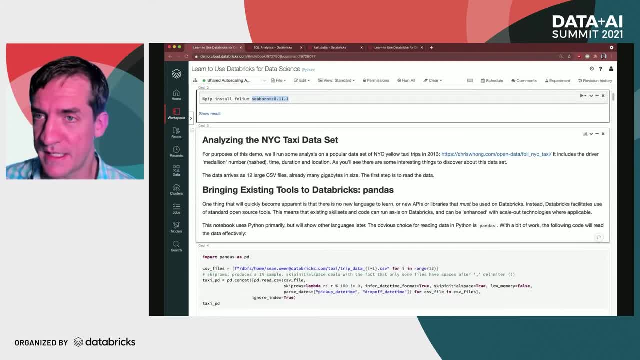 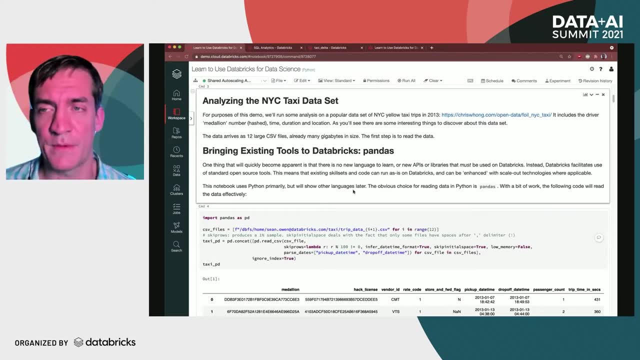 So let's have some fun with some data here. I've chosen a data set here about New York City taxi rides in 2013.. There's a couple of these data sets floating around. I picked one that I like here And it's not a complicated data set, but I think we can actually have a fair bit of fun with it. 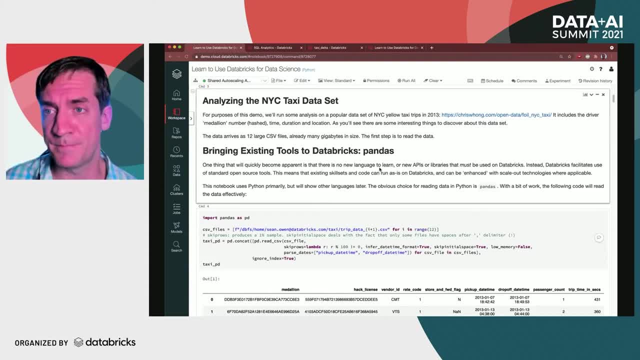 There's actually a fair bit to see even in this simple data set. So this session is oriented towards users that are maybe a little bit new to Databricks, maybe coming from an environment where they're using Python or R on a single machine and are wondering: well, how is Databricks different? 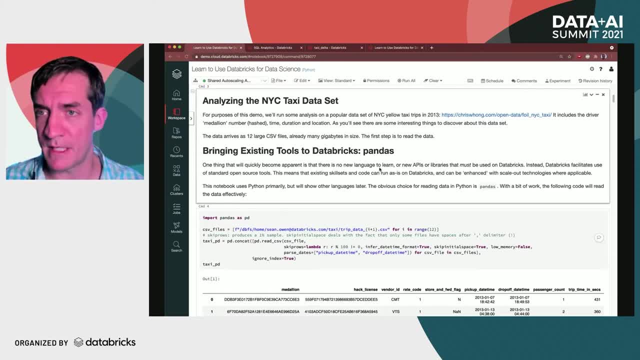 Do I have to change how I work? What does Databricks provide for me? My first message to you, starting with the Python users, is that you really don't have to change your workflow if you don't want to. So one of the first things you might do if you're a Python user is take this data set. 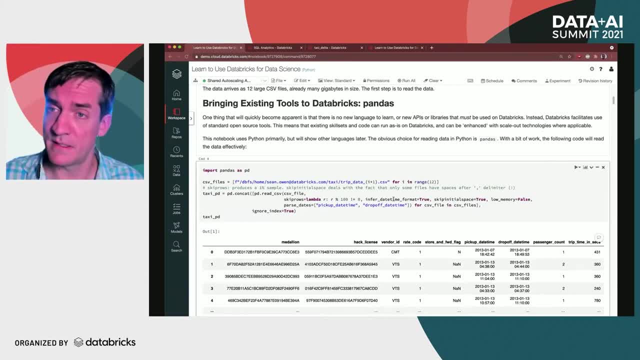 which is a bunch of CSV files, and read it with pandas. That's fine. You can do this exact same thing in Databricks. That's all I have to say. Thank you so much. That's what I'm going to do here. to start here: 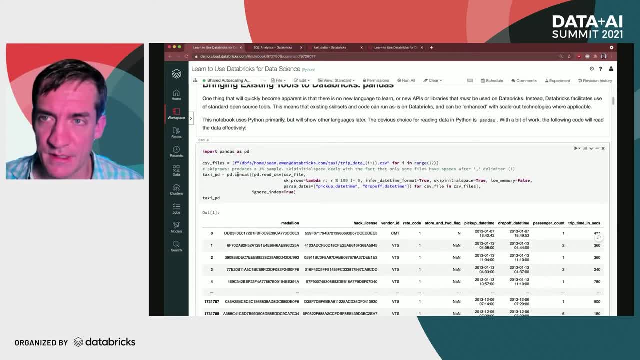 I'm going to read. there's 12 files here, So I need to put them together, And the only thing this highlights about pandas that's bad is that pandas does not distribute by itself across a cluster of machines, So it's a little bit hard to analyze. 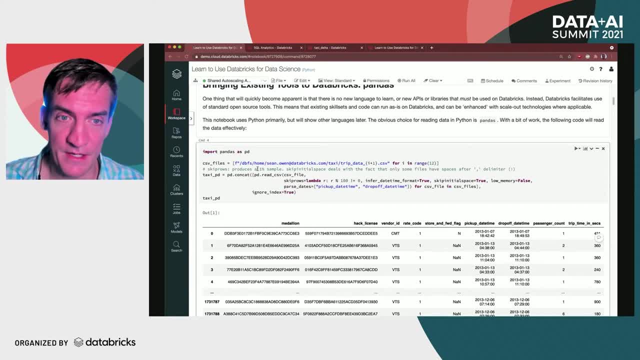 really large data sets with pandas. So you'll notice here that I've actually I've selected a 1% sample of the data. That's because the entire data set would take about 80 gigabytes to fit in the memory And maybe we could do that. 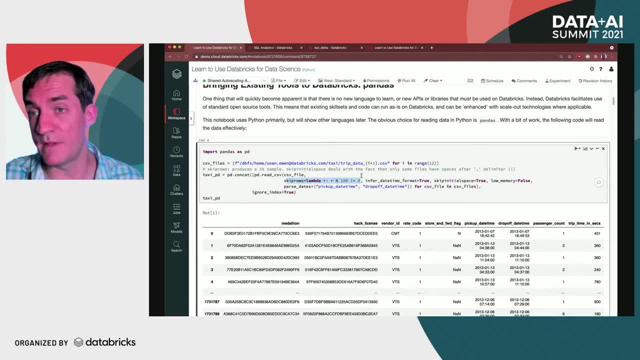 We could get a big enough machine to do that, but hey, this wouldn't really work if the data set was a terabyte, right. But fine, I mean, let's start with maybe what you know, what's simple, let's use pandas. 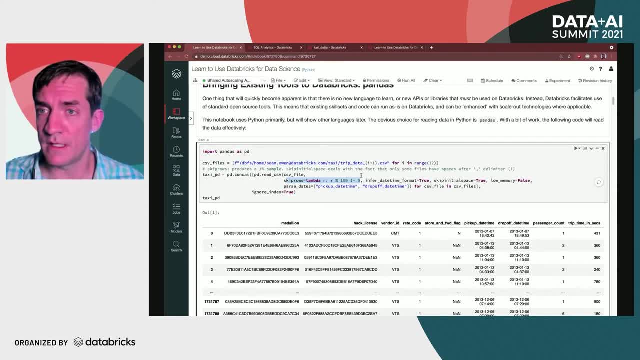 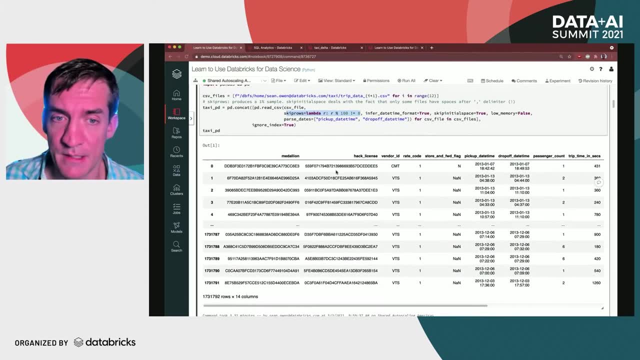 to see how far we can get with the data. So if you load a data set in pandas and Databricks, that's fine, we can do that And we can render it nicely for you here, And we see already a little bit about the data set. 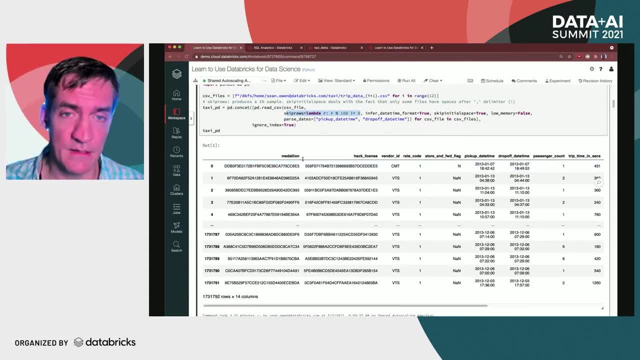 We have things like the hashed medallion and a license number of the taxi, When a particular ride started and ended, how many passengers there were, And if we scroll to the right we see it also includes things like how long it took. 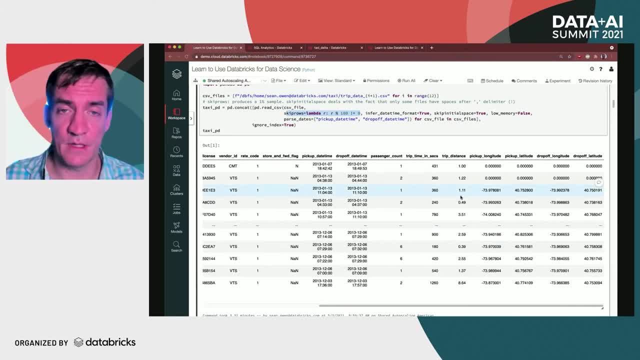 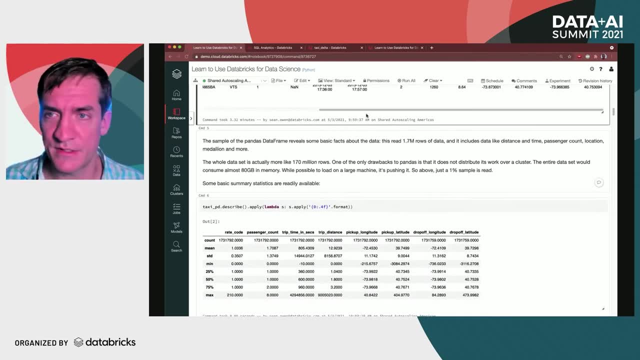 the distance and the pickup and drop off latitude and longitude Pretty interesting. There's some interesting stuff here, So any good data science process might start with just taking a look at the data. How is it distributed, And we can use pandas to describe the data. 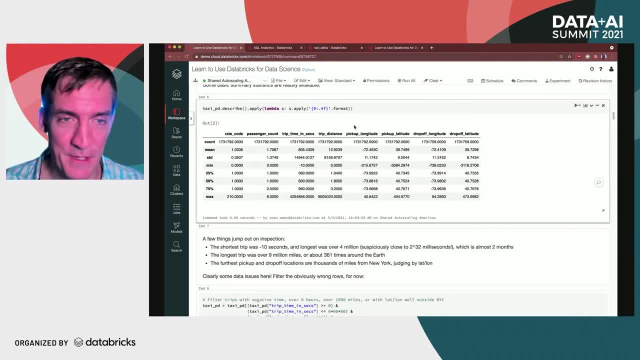 And we already see some interesting stuff here. If I may point out that, well, the minimum passenger count of any ride is zero. There were some rides that had zero passengers. I'm not really sure what to make of that. Maybe it's legitimate. 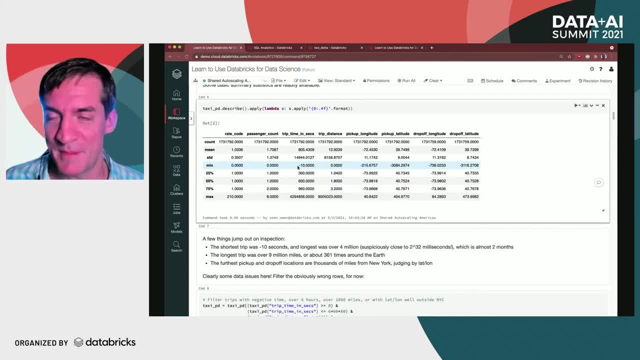 But what I won't believe is that the minimum time, the duration of a passenger of a taxi ride was negative 10 seconds. I don't think that can happen. Also, if you look at the maximum duration of a taxi ride in this data set, well, it's about two months. 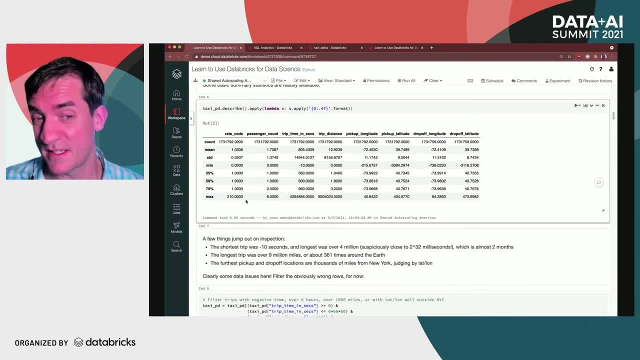 And I don't know. I've had some long taxi rides, but they weren't two months. This looks suspiciously like 2 to the 32nd millisecond, So maybe this is just a data error here. Likewise, if you look at the distance, 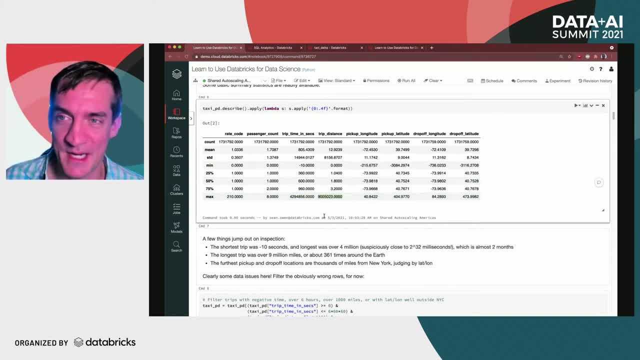 there's one trip in the data set of 9 million miles. That's about 360 times around the Earth. So I think that's probably wrong. And if you look at latitude and longitude as well, latitude can only be plus or minus 90.. Longitude can only be plus or minus 180.. So some of these minimums are obviously wrong And even putting that aside, Some of the points in this data set, these pickup and drop off points are nowhere near New York City And I've known people that have taken taxis. 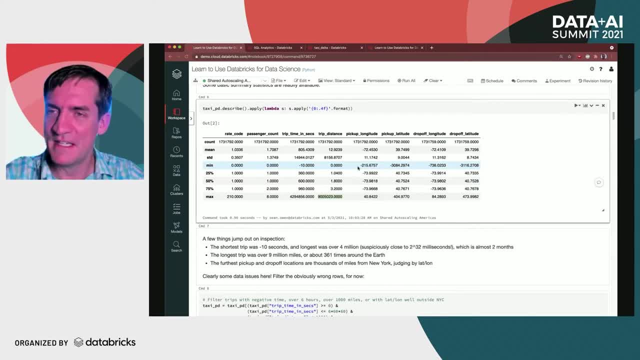 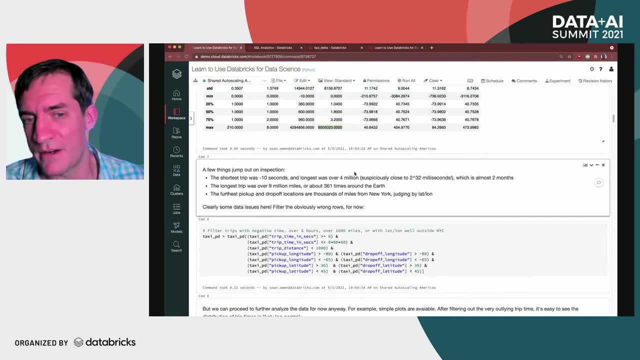 for hundreds of miles outside of New York, but probably not thousands of miles. So there's obviously some problems with this data set. As a Pandas user, you might begin by just filtering out the data points that are obviously wrong. We can do that in Pandas, right. 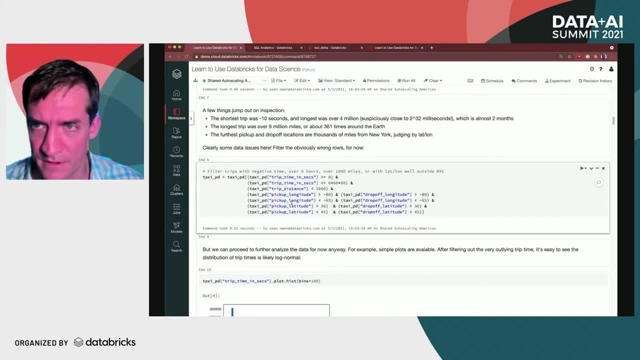 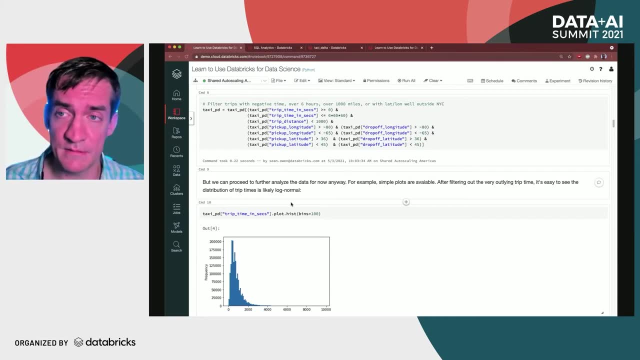 No problem here And having done that, we can start to explore the data further. So, for example, I think Pandas users will know that it integrates nicely with Matplot. it provides some nice plotting functionality out of the box. here, And maybe I want to take a look at this trip time in seconds. 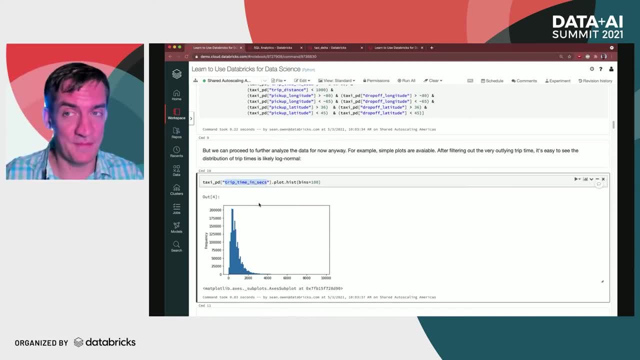 I think this is going to be a key column in the data that I want to look at more. Maybe this is the business question I'm interested in exploring, Like: what does trip time in seconds look like? How long are taxi trips on average? 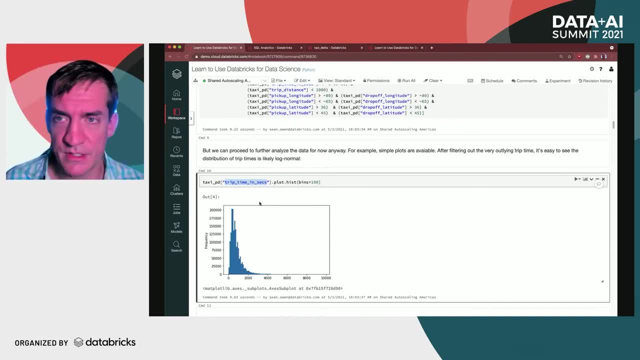 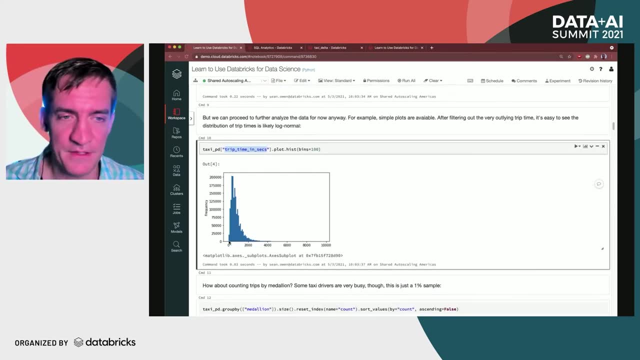 So we might start exploring that by plotting the distribution of this from my sample, from the sample I've loaded with Pandas here, And it makes some sense, I think, Obviously. OK, fine, Having filtered out the negative values, none of them are negative. 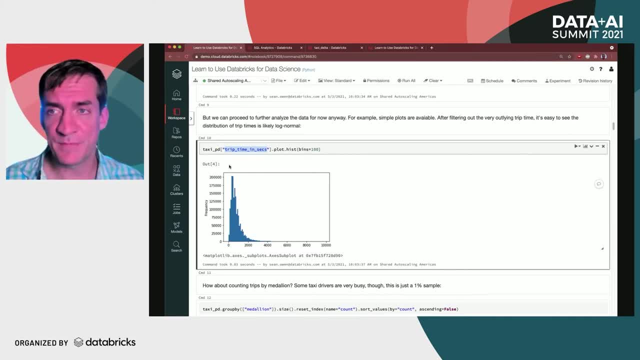 And this distribution looks log normal to me, So maybe later on I'm going to fit a distribution to that And if you're noticing some weird peaks here, well, I'll come back to that later. There's something going on with this data set. 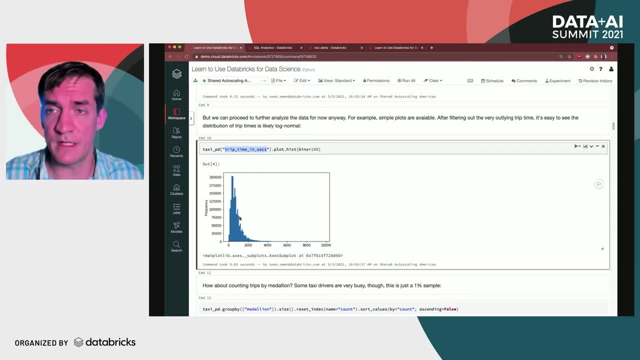 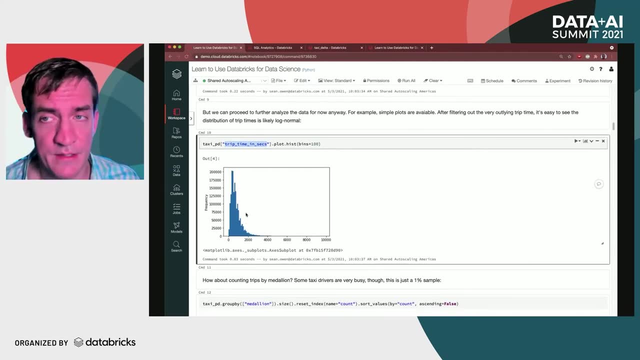 But maybe this is the key feature of the data that I'm interested in as a business user: How long are taxi trips in general? But sure, all the things you're used to using in Pandas work as well And Databricks, so no problem there. 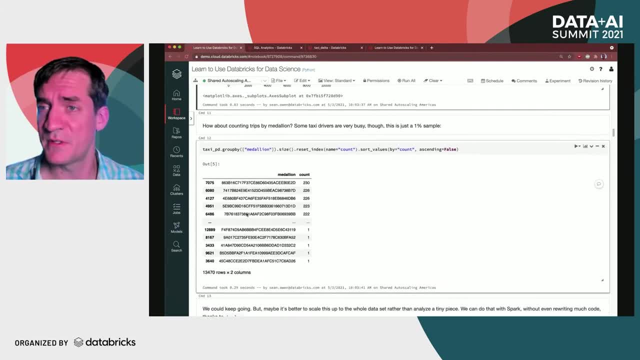 We might also want to figure out which of the taxis are most busy. So taxis are identified by a medallion. If you've been in New York City, you'll know that taxis have this alphanumeric code on top of them, like 3Y90.. 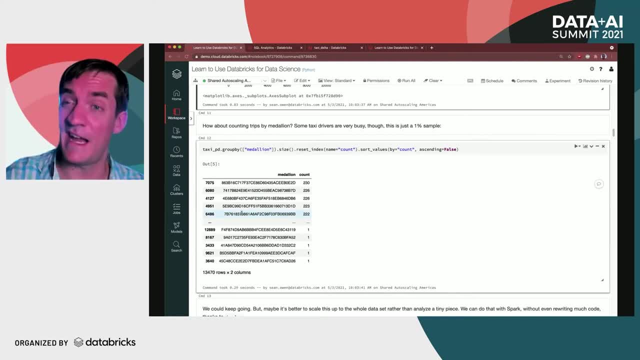 And those values are not present in the data set. They're hashed here, So we have the hash of the medallion, But we can still, of course, aggregate over that value and see which taxis in New York City are providing the most rides here. 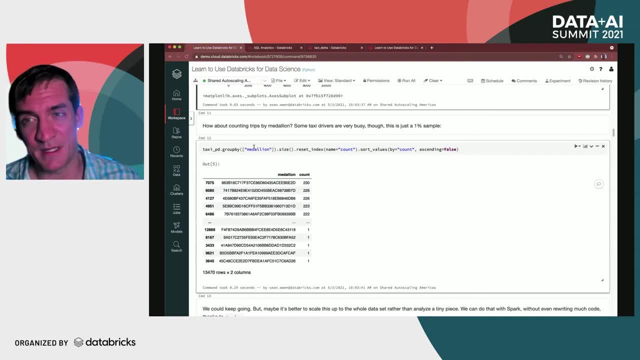 We can do that this way, But it's a little bit unsatisfying because of course, this is just a sample, So these counts are not accurate. We've just sampled 1% of the data And we counted this medallion was the most busy one according to the sample. 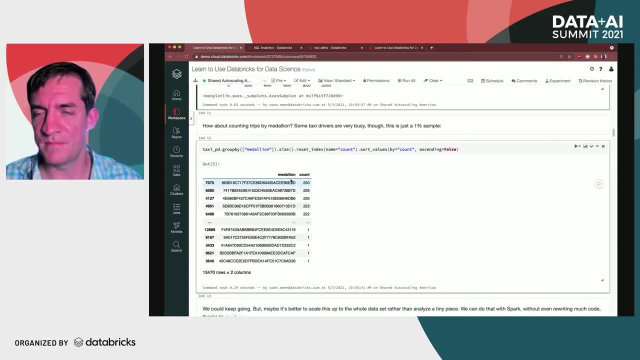 But if we're going to go further than this, maybe we want to up our game and look at the whole data set, And we can do that. We can do that. We have a cluster of machines available here in Databricks with Spark. 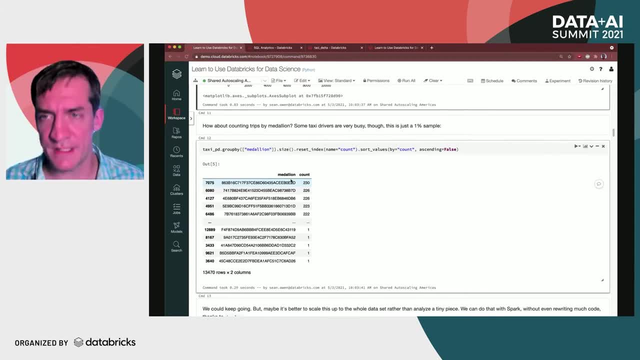 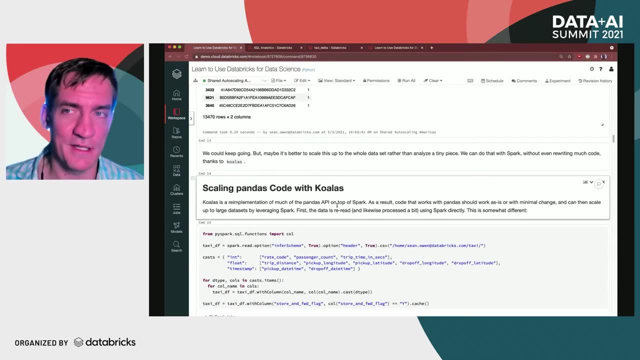 So why don't we switch gears a little bit and see what we can do to analyze the whole data set Without hitting the limitations of something like pandas? Well, that's where a tool like Koalas comes in. So you're a pandas user. 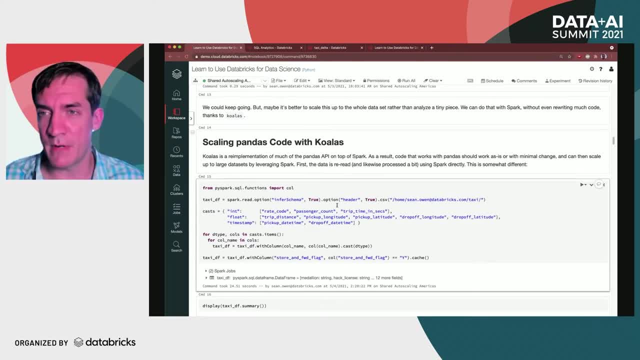 You maybe have a bunch of pandas code you've already written. You don't want to rewrite it. Of course, we can rewrite a lot of these operations in terms of PySpark, which has a similar but different API, But maybe you don't want to do that. 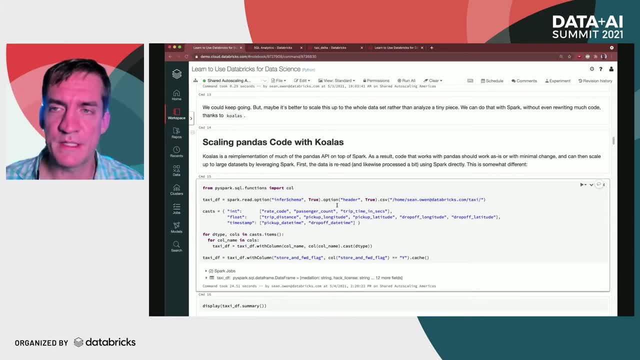 You don't want to learn PySpark. That's where Koalas comes in, And Koalas is a reimplementation of most of the pandas API on top of Spark. So that exact same code we've been executing, we can execute through Koalas, through Spark, on the entire data set. 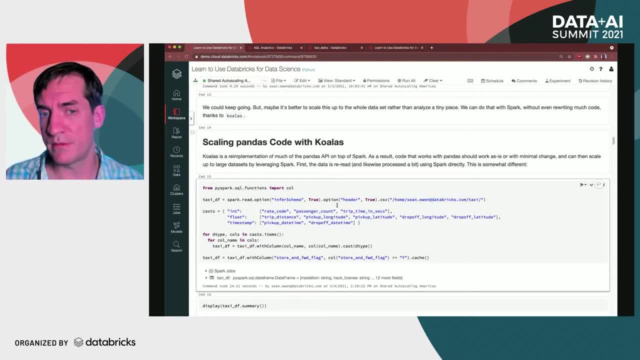 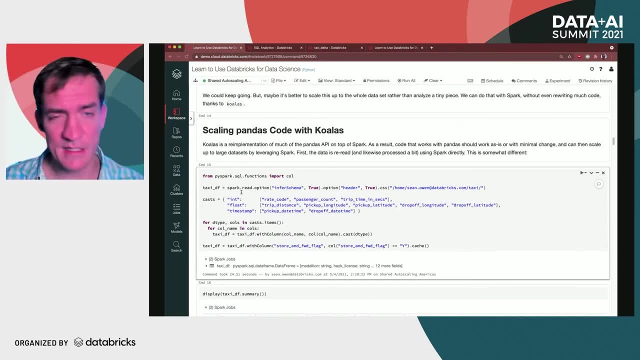 That's actually about 80 or so gigabytes, with really no change to our code. Now, the one thing that does change: yes, we have to read the data a little bit differently. Here I'm reading it directly with Spark. That's a little bit simpler. 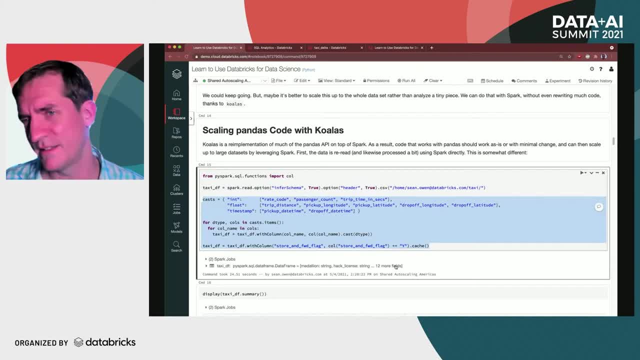 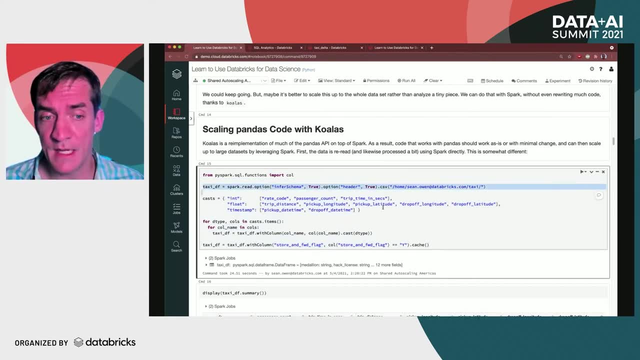 And I've thrown in some casting just to make the data look a little bit nicer. This is not strictly necessary, But I did it just to make the example work better. But we've read the data with Spark here And having read the data with Spark, well we can of course, 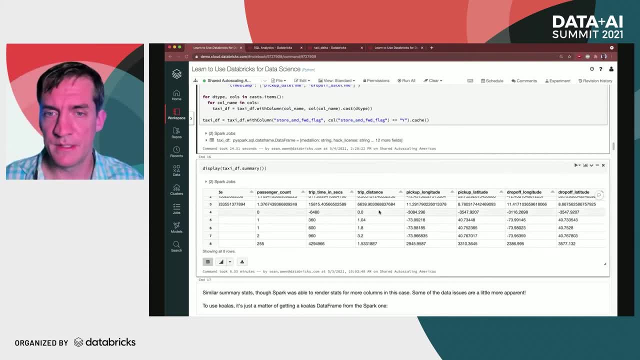 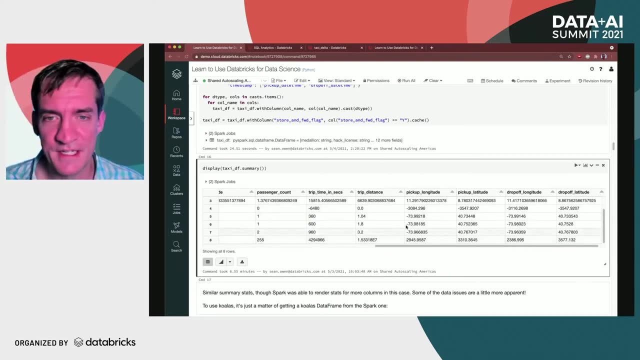 do the same sorts of things. We can call the Spark version of the scribe to summarize the data, And if we look at the summary it's a little bit different. It gives us similar ideas though, For example the apparent minimum trip time in seconds. 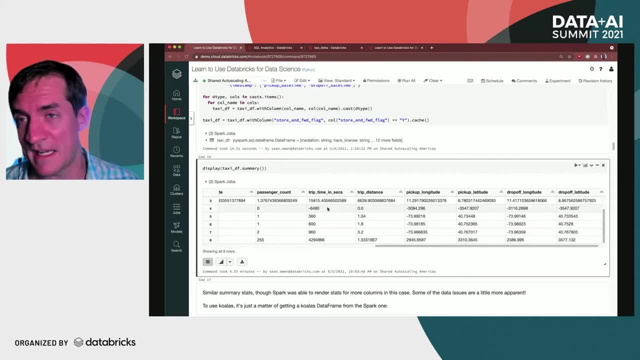 is not just minus 10 seconds, but minus 6,480 seconds, or almost two hours. So I don't know what's going on there, but someone's gone back in time. So if you look at the whole data set, you can even see more outliers here. 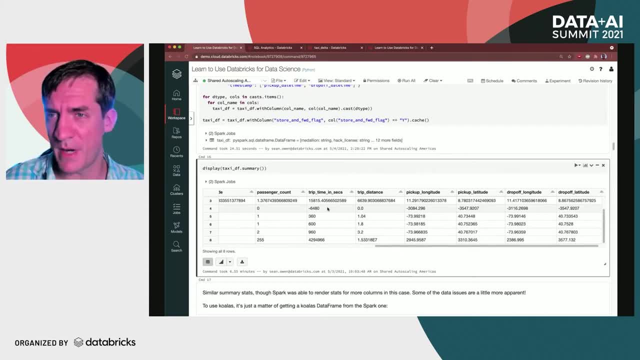 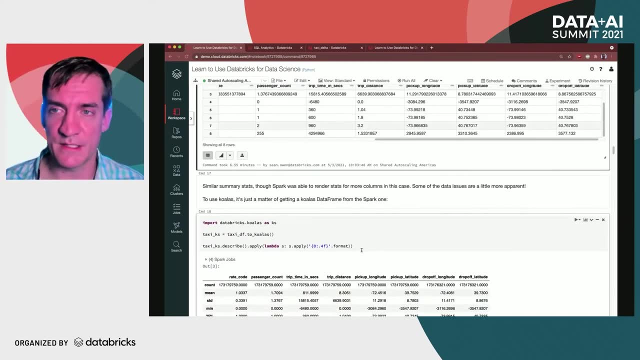 But, as I promised, maybe we want to do this work, but without rewriting a bunch of code and understanding the PySpark APIs. So let's use Koalas to actually do the exact same analysis that we did above. So here I'm, transforming this Spark data frame into a Koalas data frame. 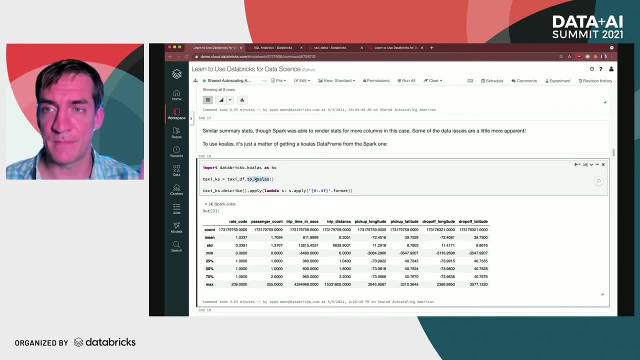 It's a wrapper on top of the Spark data frame that gives us methods and syntax that work like pandas, So this is the exact same line of code. I executed above on this pandas sample of the data And it works as well. So now I'm executing over, however, the entire data set. 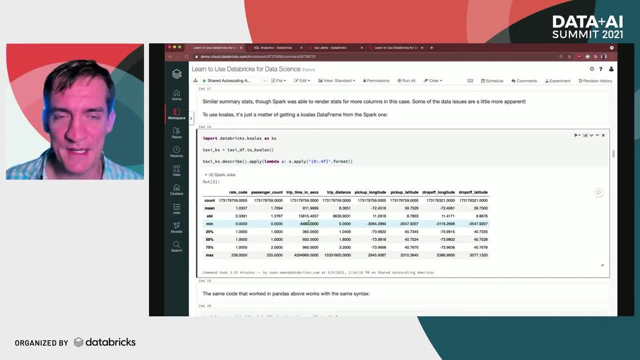 And indeed I see the same sorts of interesting artifacts. The worst trip time in seconds is much smaller. And boy, some of these longitudes and latitudes are really quite crazy here. But we can execute the same code to filter it here. 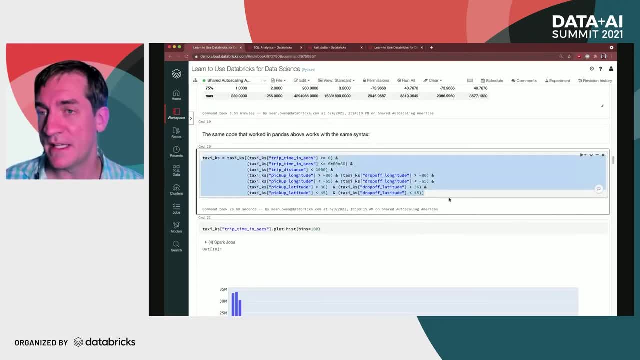 This is again, I assure you, the exact same code I showed you above. This is pandas syntax, but it's implemented in terms of Koalas. So this happens across a cluster, on the entire data set, And we can also render a plot, a histogram of that trip time. 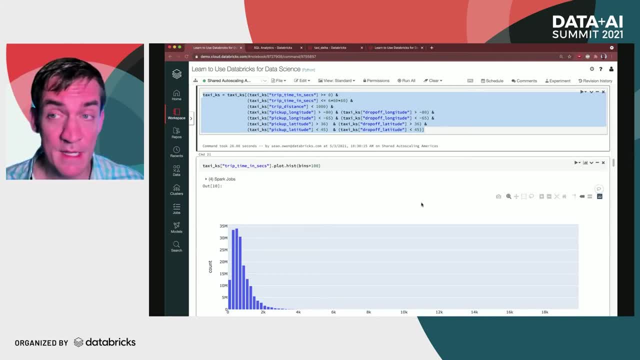 in seconds, which is one of the key features we're interested in Now in Databricks. if you do this, even though Koalas is open source and you can use it anywhere else, like a lot of open source things- 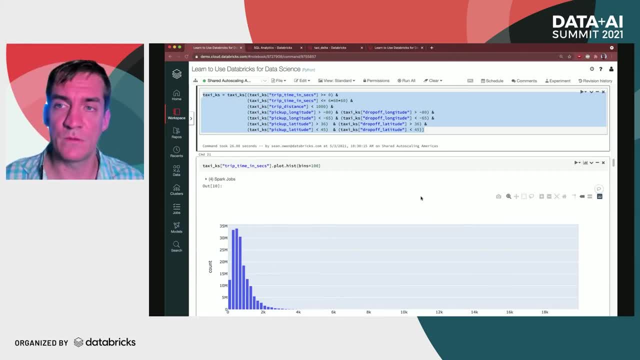 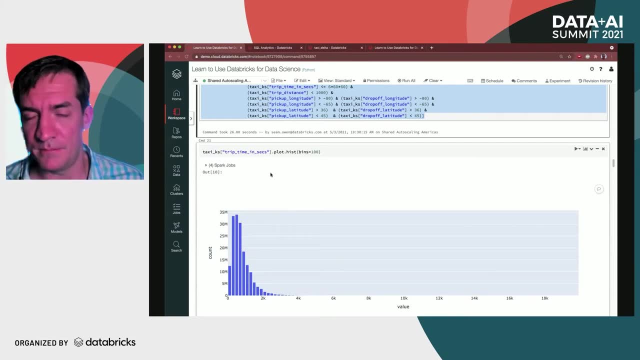 we can make Koalas run a little bit better in Databricks, And so in Databricks if you plot something with Koalas, we can detect that and render a nicer plotly-based histogram from this data. So you'll see, this is actually a little bit in a different way. 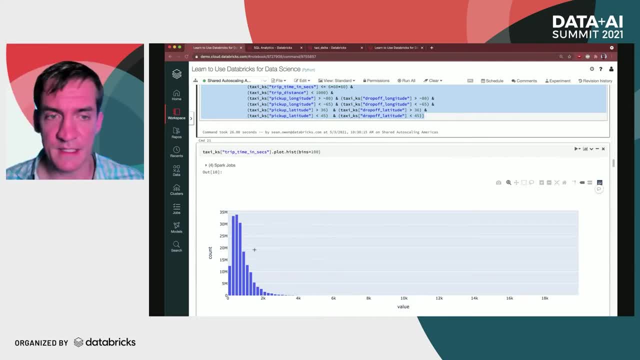 It's a little bit more interactive here and I can mouse over the data set and explore it a little bit more. And the nice thing is we're actually looking at the histogram of the whole data set, So maybe we can have a little more confidence. 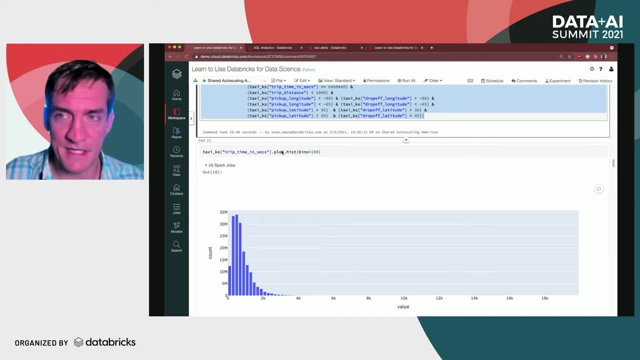 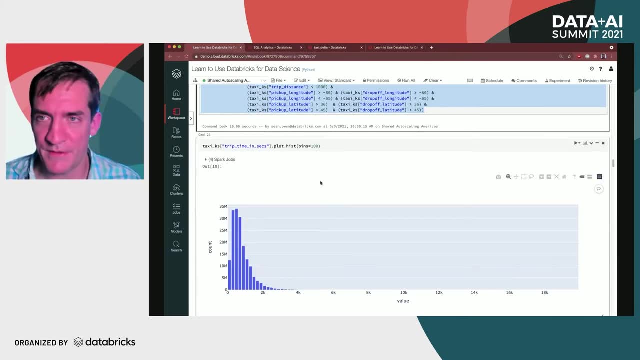 in that what we're looking at is the true distribution, But I'll tell you that something interesting emerges. if you make this histogram a little more fine grained- Because we have the whole data set- we can do this and see something more interesting. 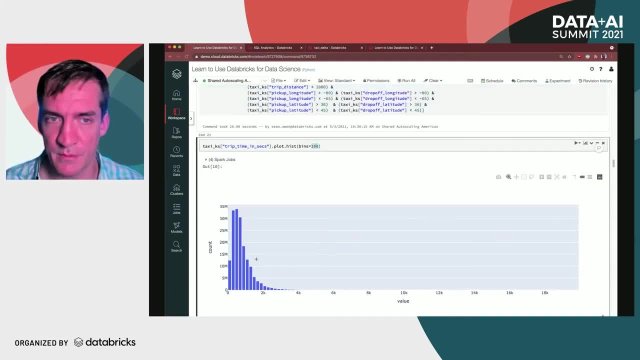 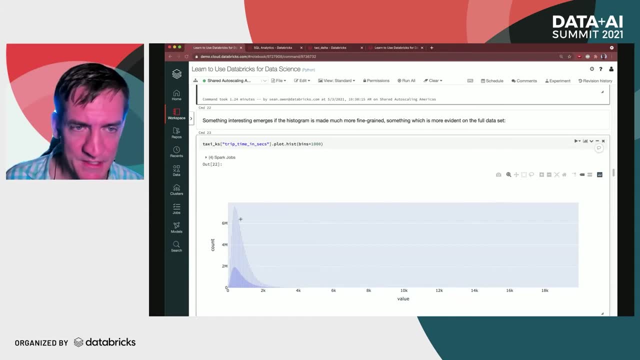 What if I upped this to 1,000 to slice these bins a little more finely? Well, this happens here. So you see that there's actually two distributions going on. Let me zoom in on this. Yeah, so this distribution of frequencies of trip times in seconds. 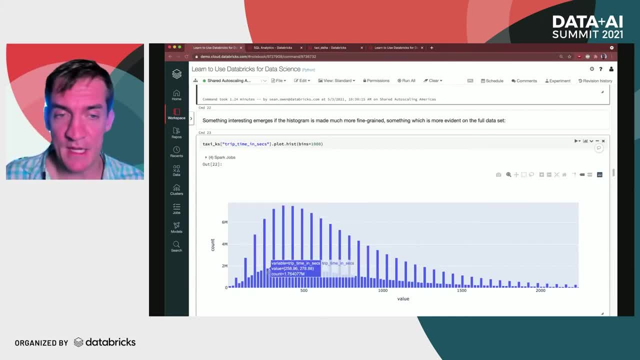 has these very clear and regular peaks And if you look closely, you'll find that these peaks occur at multiples of 60 seconds or one minute. So if you spend a lot of time in New York, like I did before 2013,. 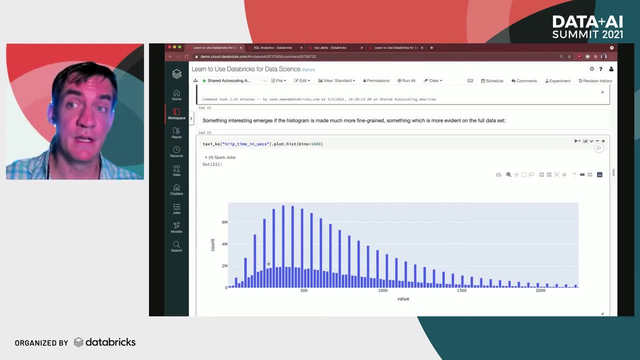 you may think that, yes, New York City taxis measure their time and their fares in terms of minutes. Maybe newer ones can measure them down to the second and build at the second. I'm not sure, But this is quite apparent from the data. 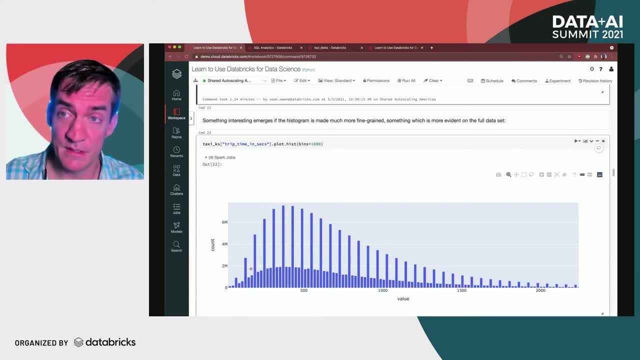 A lot of this data seems to be reported with this trip time feature, quantized to the nearest 60 seconds or so, And that becomes obvious if you can plot this And hey, that's an example of data science. But given the tools, given easy tools to look at the data, 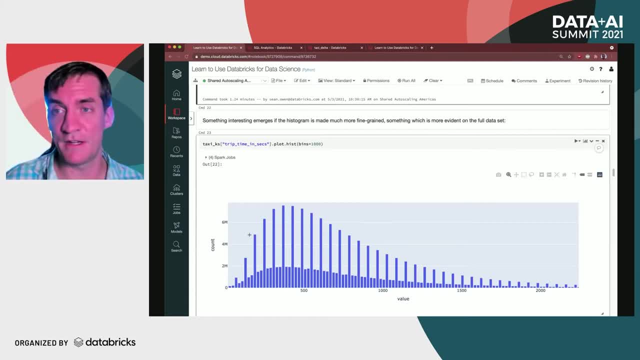 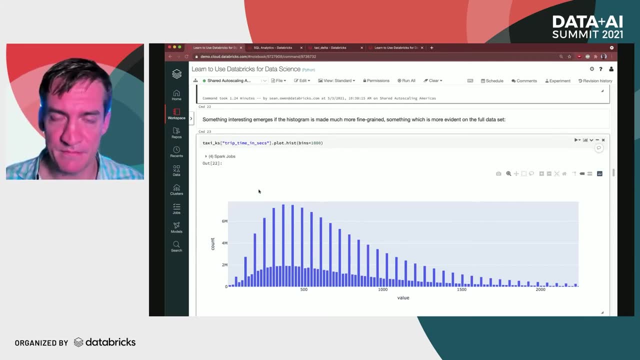 we can see these things and at least work around them, or, if we need to go upstream and fix them. But yes, let's be aware that this column, yes, the data is good in the main, but a lot of it is rounded to the nearest 60 seconds, obviously. 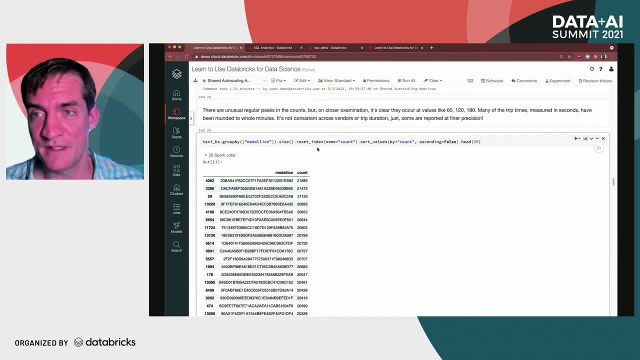 So we can go back and do the same thing again, same Pandas code executed through Koalas across the entire data set. So we can efficiently do counts by medallion here over the whole data set And we see that, yeah, some medallions, some taxi numbers. 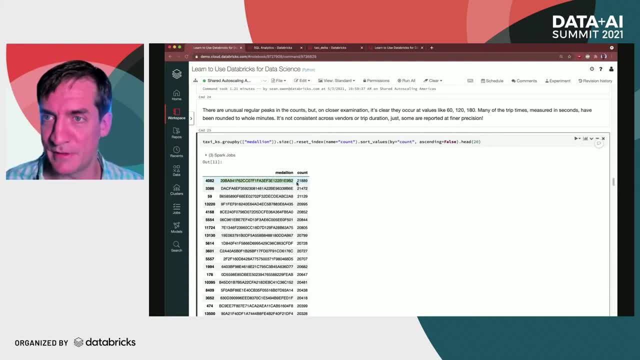 were really quite busy in 2013.. In fact, I'm not sure I believe it. Apparently, one taxi medallion delivered almost 22,000 trips in 2013.. If you do the math, that's about 60 a day. 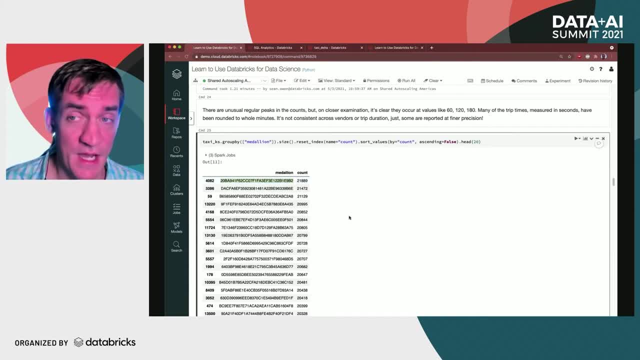 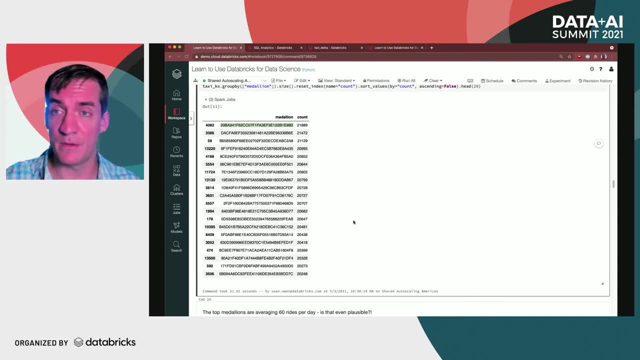 That's 5 an hour for a 12-hour day. That seems kind of unlikely And I won't show it here. but I went and broke this down further by license and medallion both at the same time, And you still come up with a maximum that's really quite high. 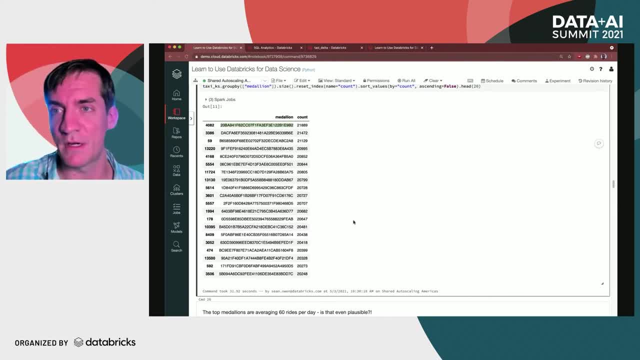 So I'm not sure what's going on there Maybe. So this is a New York City Taxi and Limousine Commission. You might look at some of these to see if people maybe are several different distinct people are sharing a medallion or a taxi license. 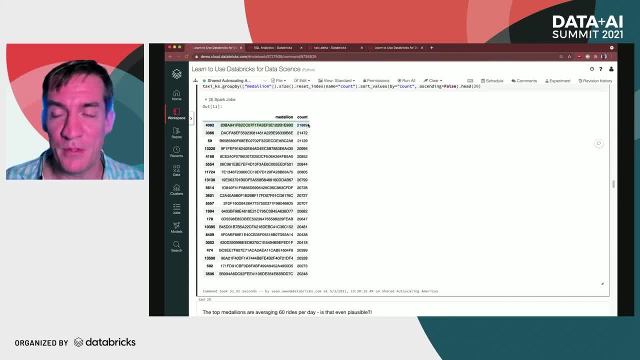 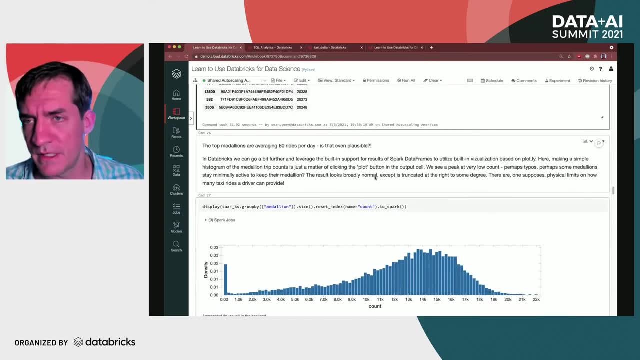 I'm not even sure that's a problem or not, But this seems pushing the bounds of what is physically possible for taxis in New York City. And we can also, if we like, flipped on the built-in visualization in Databricks which I've shown you a little bit above. 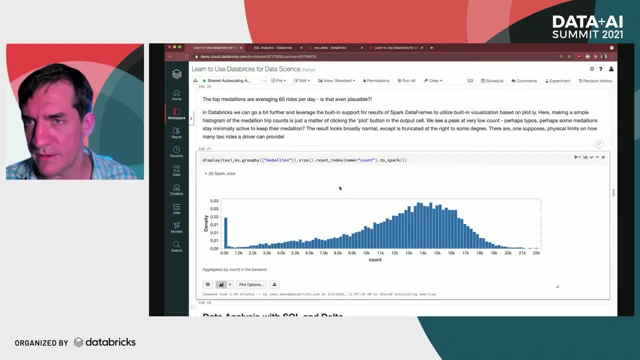 to plot this data- Again, another history- We don't have to use other tools. We can just access these plot-based visualizations in Databricks if we just want to take a quick look at the data. And so if I plot the distribution of rides, 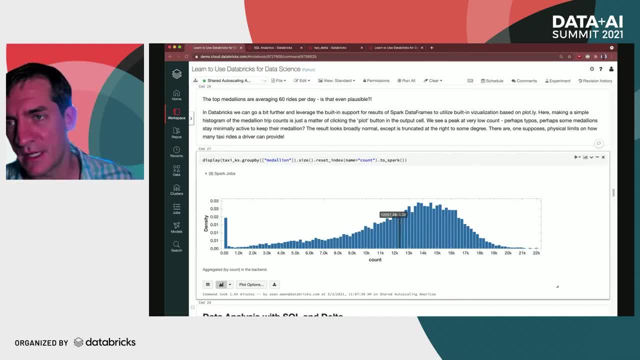 by medallion in the counts. well, I see this distribution. that's normal-ish, But obviously it's truncated at the right because there are physical limits on how many rides a taxi can possibly provide in a year. But you also see this nice peak at the left here. 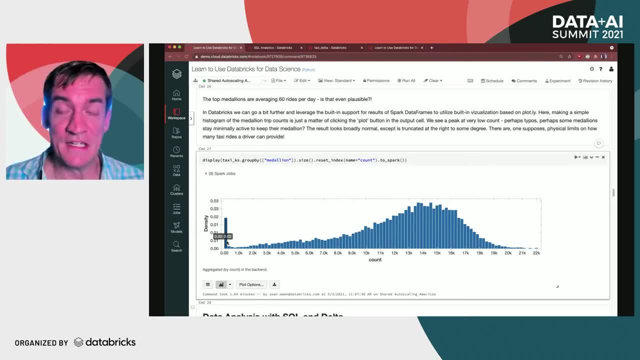 And this is not 0. This is 1 if you look at the data. So why might that be? Well, I'm thinking that maybe there are rules that say, if you don't use your medallion at least once a year, you lose it. 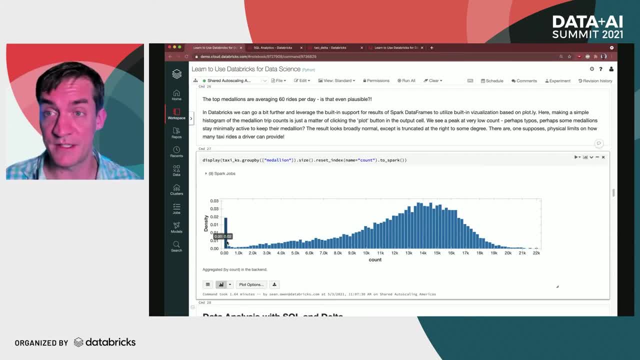 So maybe there's some incentive for a lot of taxi medallions to take a ride at least once a year, and only once a year, And so maybe that's what's going on here. I don't know, But if I were a data scientist and I were exploring this data on behalf of New York, 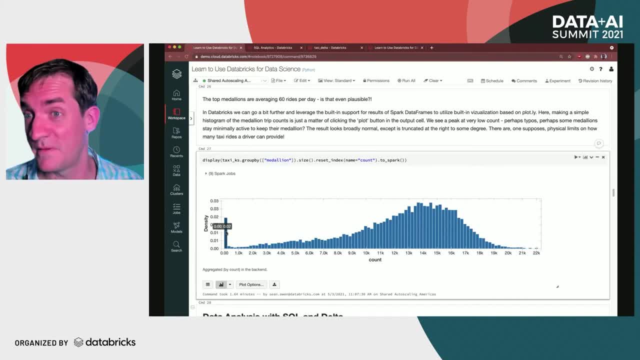 City, then maybe these medallions would be of quite a bit of interest to me And it's nice that I can see that pretty easily. But I think it's a great tool to use by querying the data and firing up a quick visualization. 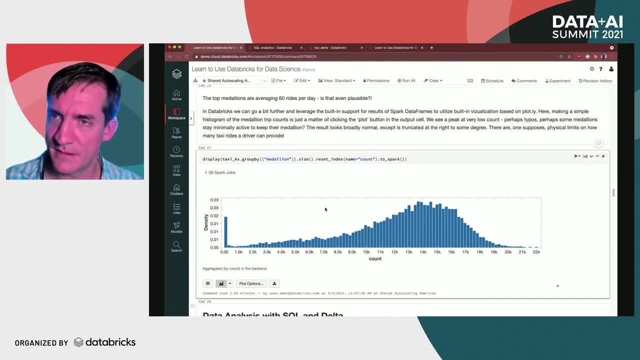 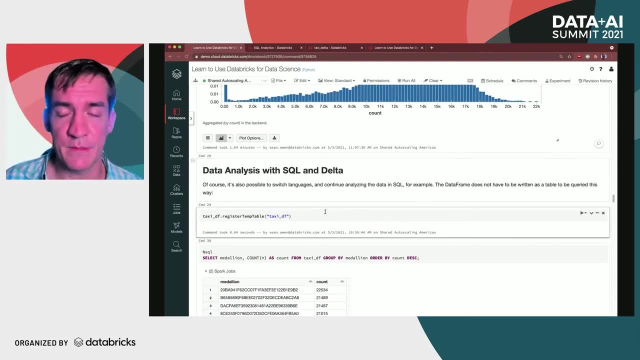 of it. So, moving on, I think I've addressed the Python users here, But of course, I think a lot of people in the audience are probably SQL users as well. They're used to querying data with SQL and they may be wondering what does this tool? 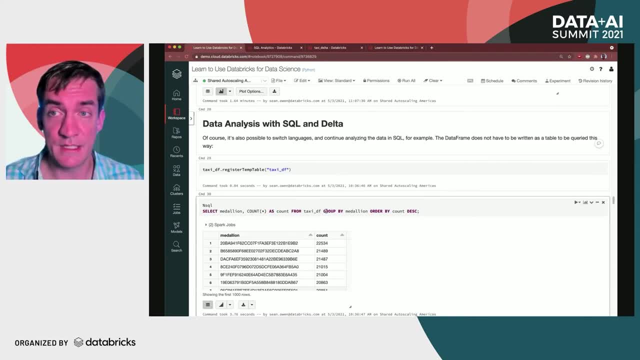 have for me. Well, the good news is, of course, you can query data in SQL and Databricks as well, I think. as Austin alluded to, Databricks has an entire BI language, So I'm not going to show you here. 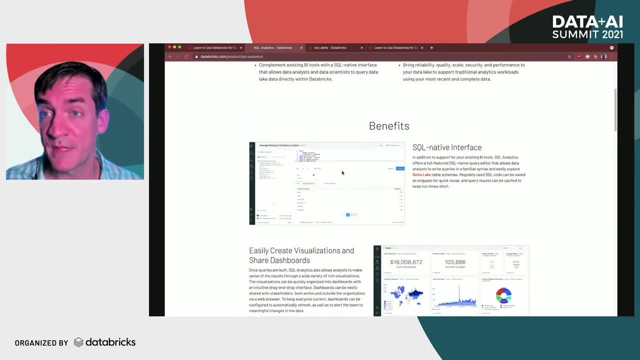 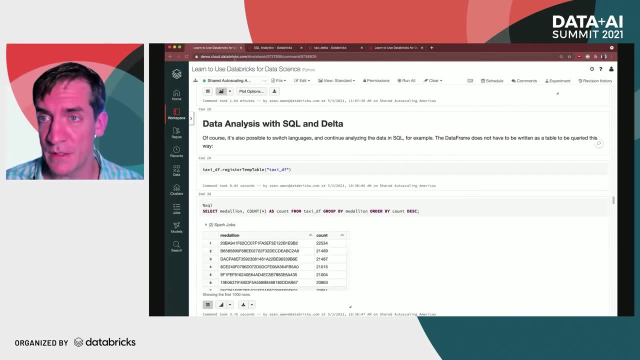 I'll give you a quick peek at it here from our documentation. So rest assured that if you're a SQL user and want a BI-like environment, we have that in Databricks. But I want to show you here that you can do that inline in a notebook as well. 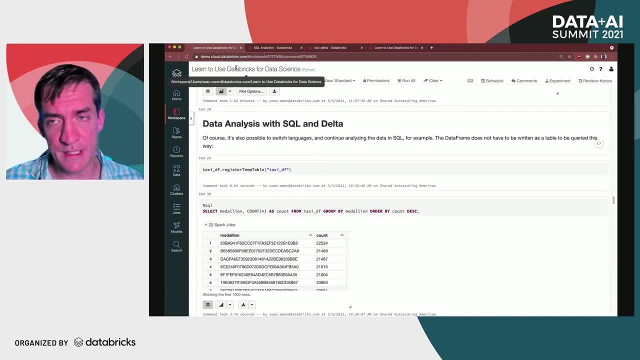 So I've been querying data with Spark, maybe via Koalas here, But if I like I can switch to SQL or a different language even within the same notebook, And I'm going to switch to SQL here to query this data frame. 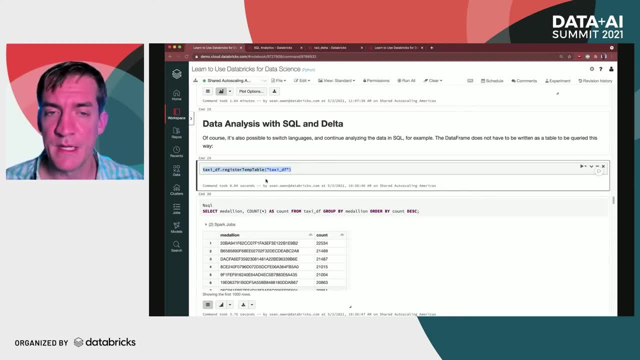 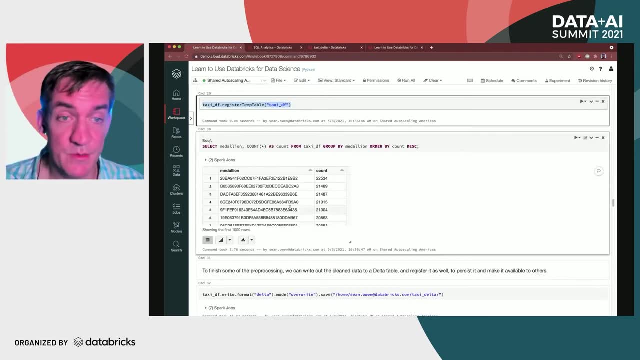 This Spark result that I've been forming here, And I can do exactly the same things if SQL is a more comfortable language to express the queries you want. So here I am, issuing the same query: Show me the count of rides by medallion. 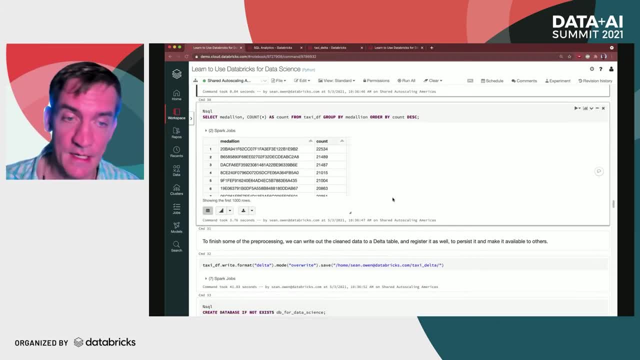 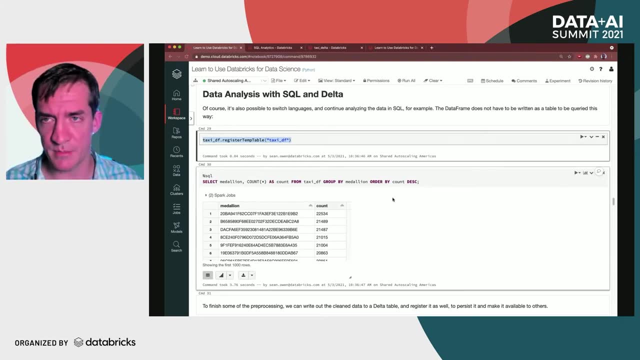 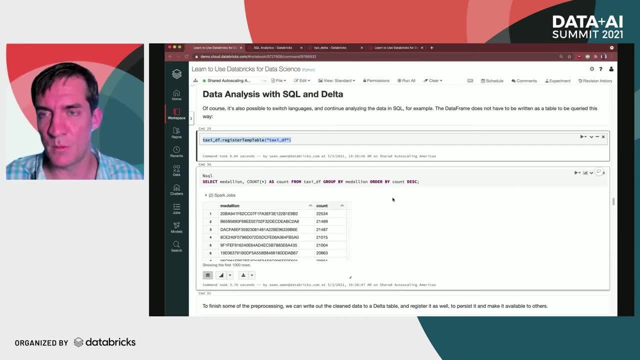 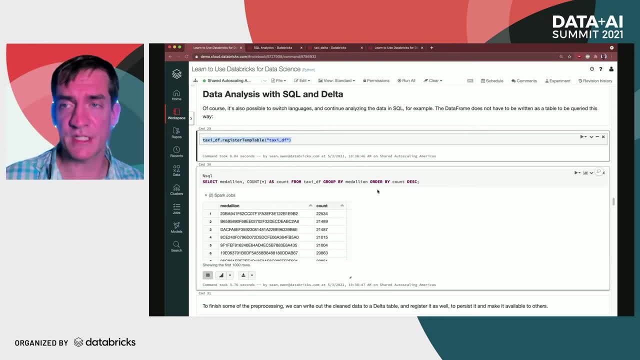 It's just a Spark data frame. It's the result of transformations I've expressed with Spark. But if I like I could persist that result to disk, to distributed storage in your storage account and then register that data set as a table in a database. 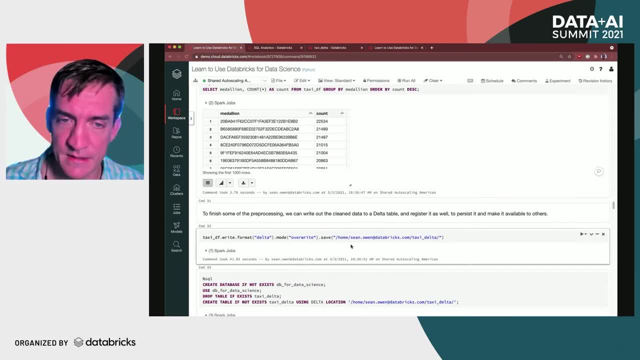 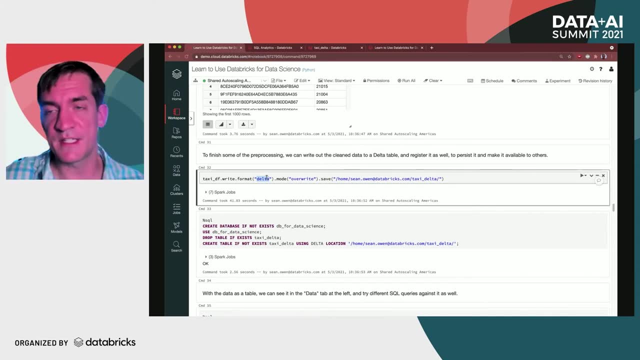 So that's what I'm doing here: I'm going to save this. I'm going to save this data set as a Delta table. Delta is an open source storage engine from Databricks And it builds on Parquet to add some additional features like merges, upserts, deletes, transactions. 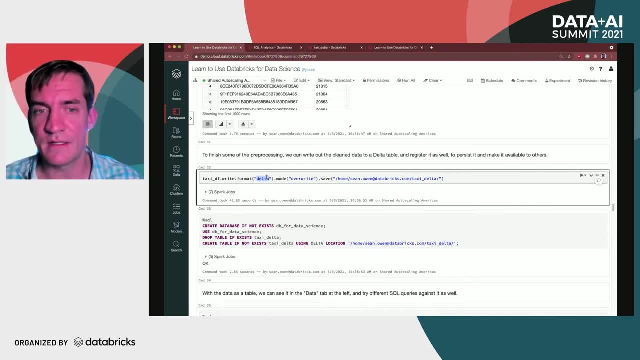 and time travel to let you query the state of the data at a previous point in time. So it's a good choice, I think. if you're working in Databricks- But you really don't have to- You could save these as Parquet files, as agro files, JSON. 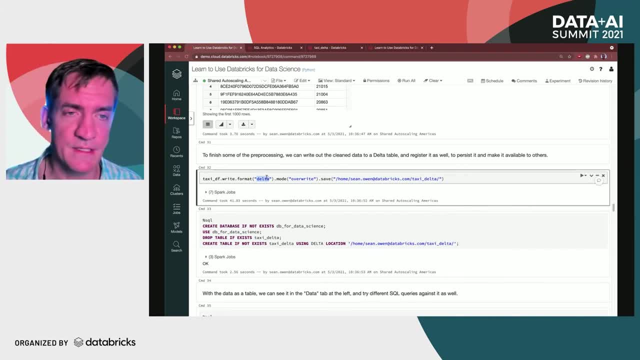 It really doesn't matter. You can read or write anything Databricks. But I've written this as Delta And I'm going to register this table as a table in the Metastore here. that's built into Databricks And if I do, this becomes visible here in my Metastore. 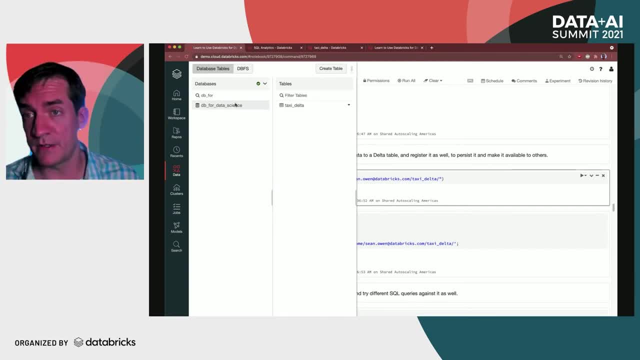 Yeah, here we go, And that helps discovery. So other people now can access this data from this database, from this table, even though it's really just files on disk and distributed storage in an open format. So for SQL users, for database users, the rest of the stuff, it's going to look like this: 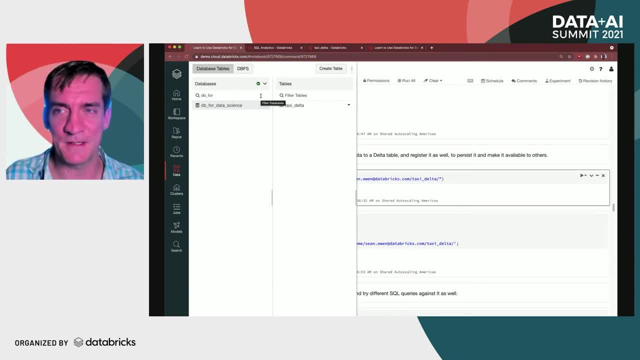 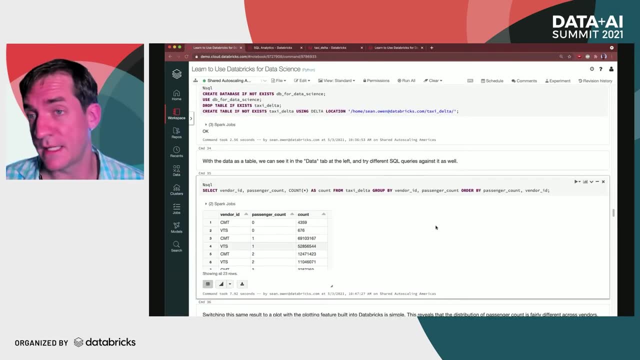 So that's kind of the whole idea here. Thank you, guys. You're welcome. You're welcome, sure you can do these things. you can still have concepts of databases and tables and data that's persistent and so on, and if i do that, of course, well, i can continue with sql here, even in line. 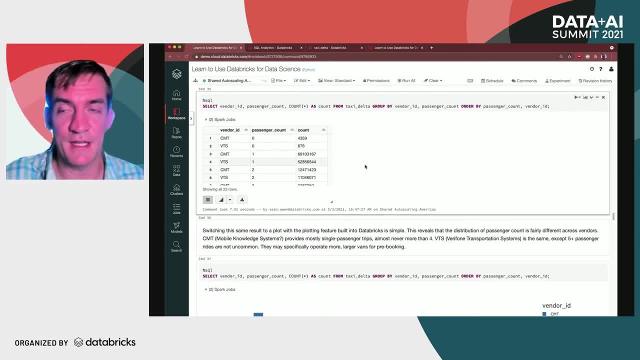 in a notebook and issue maybe different queries. maybe i'm interested in the distribution of passenger accounts across uh, across rides here. so if i break this down by vendor and passenger count, i see well, number one. strangely enough, there's quite a few rides recorded in 2013. 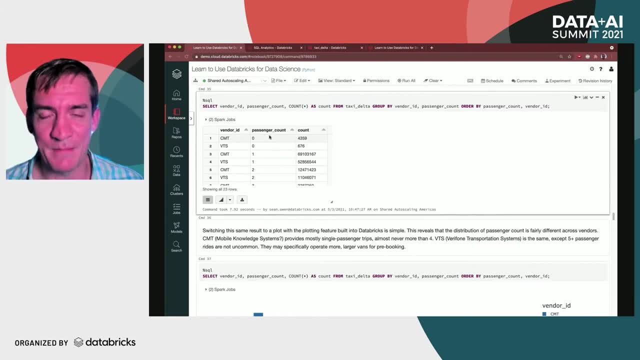 without any passengers. not really sure why that is. i'm not sure it's invalid, but i don't. i can explain that typically taxis have passengers, but i might want to break this down uh and visualize this uh by event. these counts by vendor and passenger account as well, and i can, of course, 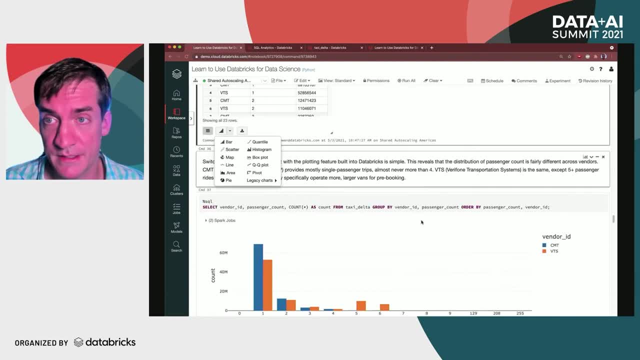 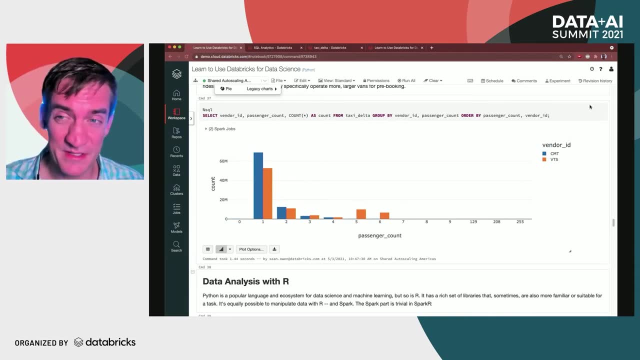 just simply flip on the built-in visualization here in databricks and i get something like this and immediately something pops out of here for these two different vendors. their distributions are different. so cmt is uh, uh, the company is called a Tokyo. Tokyo has a fixed management platform, uh, and they're mobile knowledge systems and i think. 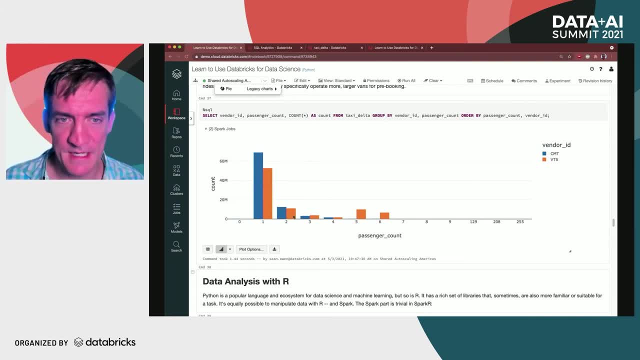 this is the company that runs the hardware for your standard new york taxis and indeed for those in blue. you see that, uh, well, as expected, most time, most of the time, taxis have one passenger, sometimes two, rarely three or four, and not really not more than that. but for uh taxis operated by 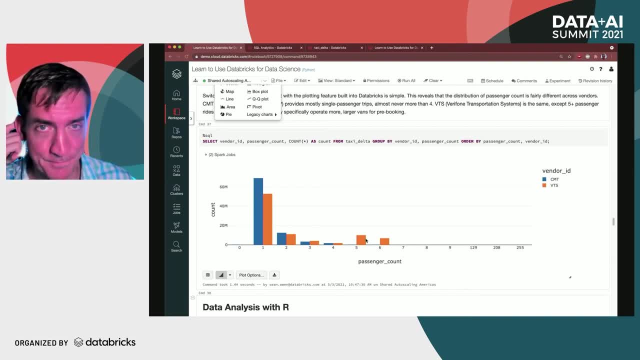 by VTS, which is verifone transportation systems. you see the spike at five and six and i think having a service where you can pre-book much larger taxis, like vans, to transport more than four people that could possibly fit comfortably in a taxi. so you know, maybe that's interesting, maybe it's not, but 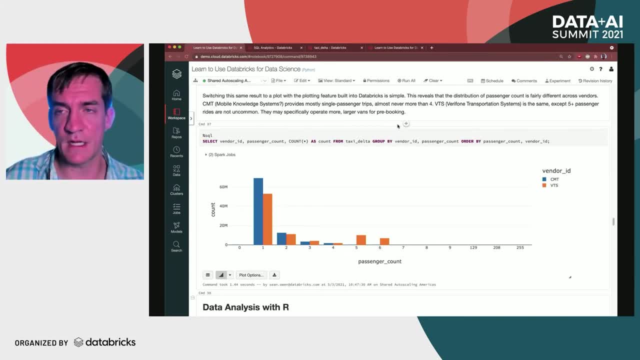 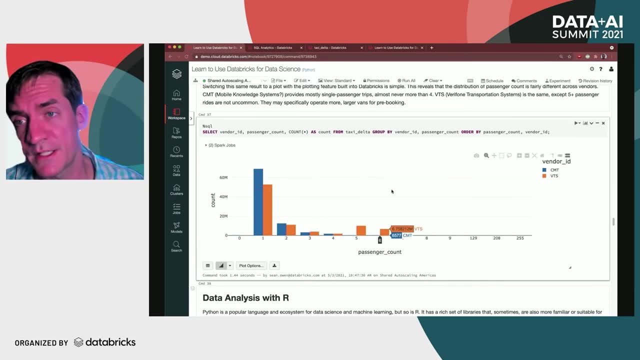 these are the kind of things that are easy to see immediately from this data set if you just load it and query it with sql and maybe plot it with built-in tools here in databricks. so let's switch languages again. i imagine there's some people in the audience who are our users are as 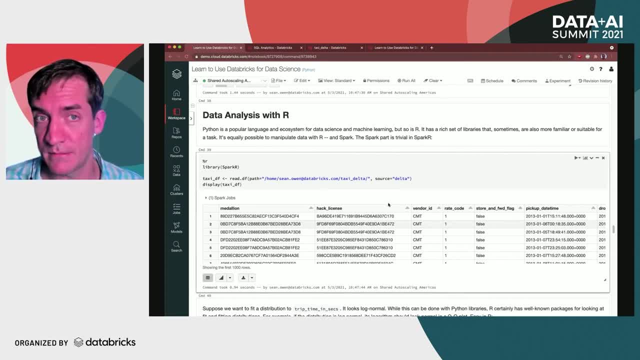 a rich statistical environment and it's a one of the tools that people might most often reach for to do more advanced statistical analysis of data. and the good news is, in databricks, r is available as well, so when you run a notebook, there is an r interpreter available as well if you wish to use. 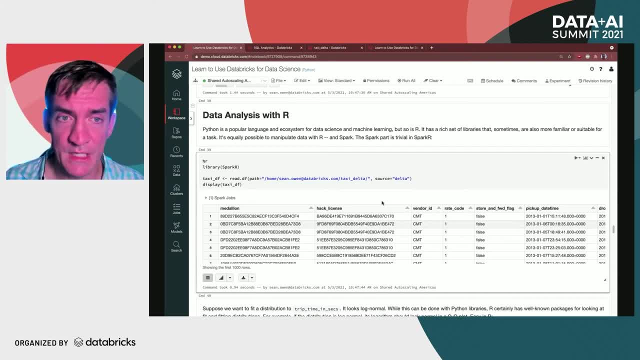 it to also create the data and transform it. so here i'm going to switch into r. i can do that within one, within a notebook, here by switching with this magic command, and i'm going to load sparkr, the library that lets me add a search button to the database. i can do that within. 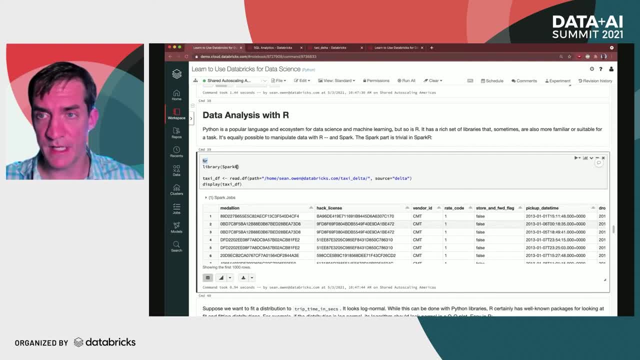 within a notebook here by switching with this magic command, and i'm going to load sparkr, the library that lets me add access data via Spark, maybe store it out there as Delta tables in R, and that's what I'm doing here, And it's really just the same thing. 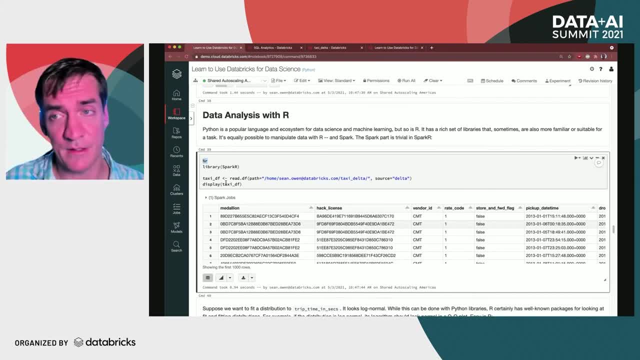 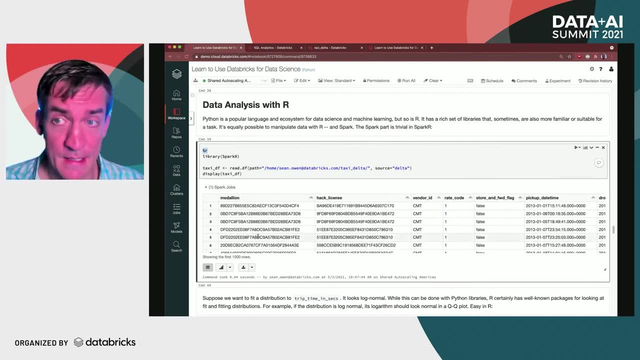 So if you're an R user, all the stuff we've been doing in Python you can do in R as well. There's equivalent libraries to manipulate the data at scale with Spark. So here's our data set. But again, as I say, I think we're interested. 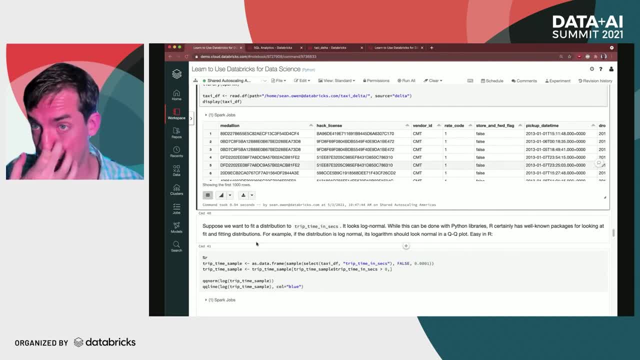 in this trip time feature. As I said above, I think it looks log normal And I want to drill down on that question. Is it actually log normal And if so, what is the log normal? distribution of trip time in seconds. Now I know how to do that in R. 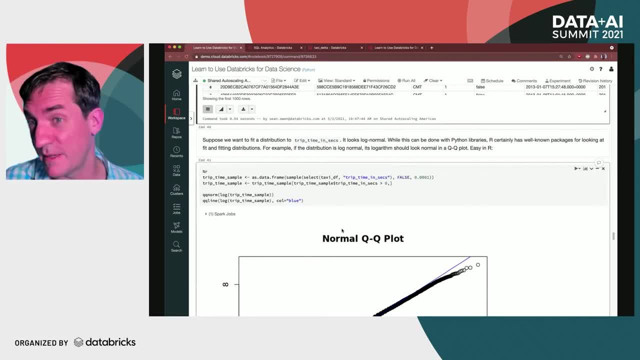 I might know how to do that in Python if I looked up the equivalent methods and stats models or something, But I definitely know how to do it in R, So why don't I just do it in R? So what I'm gonna do here is: well, again. 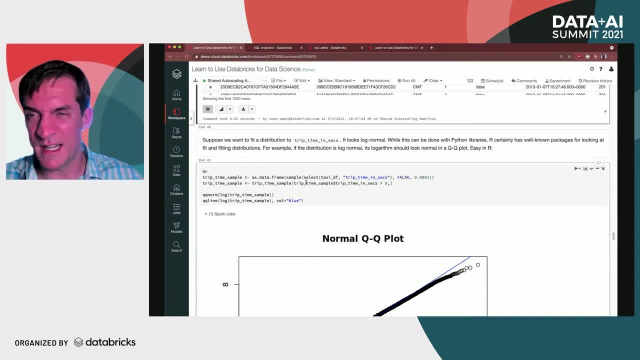 I need to take a sample of the data because we're working in R and this data set's huge So I can't bring the whole data set down. but I don't really need it to maybe look at the distribution of trip times. So I'm just gonna take a random sample with Spark. 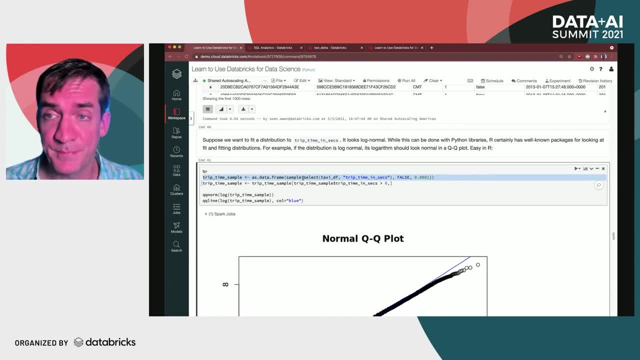 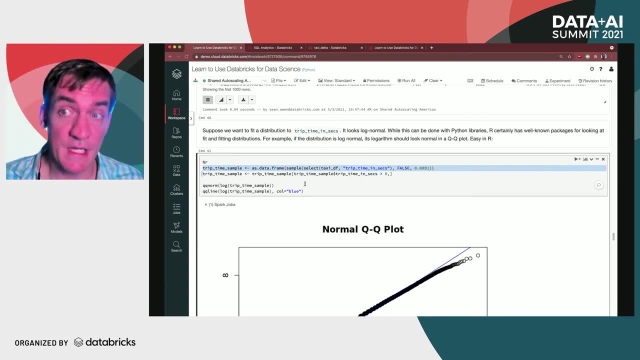 and pull that small sample down to as an R data frame And from there I can work with this data set as I would any other in R. So if the data set is log normal, then the logarithm of the data points should be normally distributed. 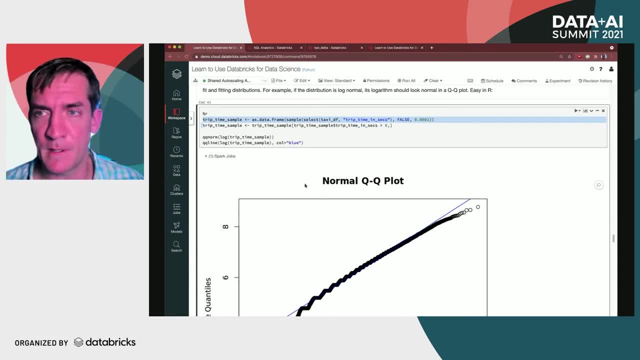 Then I can assess that with a QQplot standard stuff in R We do actually have built-in visualization for QQplots, but I wanted to show you how to do it in R, because I think a lot of users out there are probably accustomed to doing this in something like R. 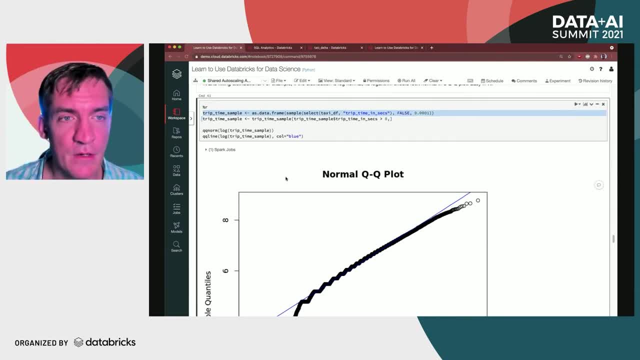 And I just want to show you that it works exactly the same way. So here I'm gonna make a QQplot of the logarithm of trip time And I'm also gonna fit the theoretical fit line for this data, so I can maybe assess whether this looks normal or not. 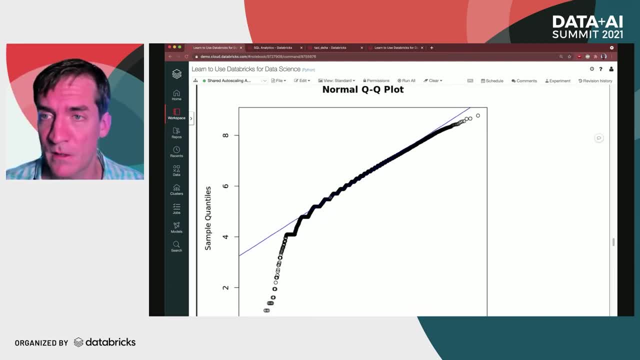 And here's what I get. It's gonna be very familiar for people that have worked in R or RStudio. I will say on the R side we do have an integration with RStudio as well for the R users. You can run RStudio in Databricks. 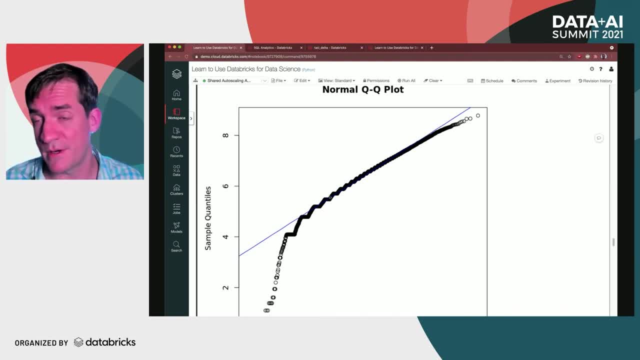 and use that with a Databricks cluster. But here I'm just using R directly in the notebook. That's fine too. And what do we see? Well, this blue line tells us what the data should look like, if it really is perfectly log, normal. 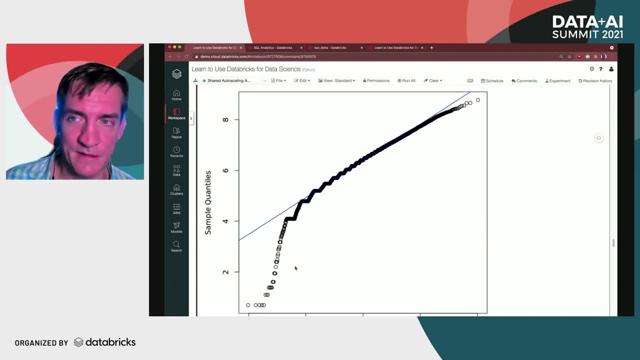 And it's not quite. It's notably light tail on the left end here, And maybe that makes sense because, well, it's probably unlikely you take a taxi ride that takes one minute or 30 seconds. So even though this distribution might predict, 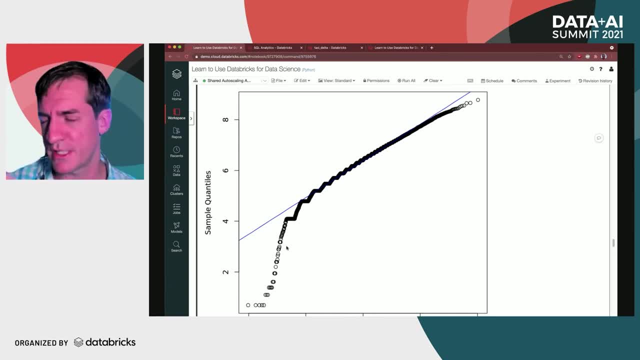 that there's some of those those are highly disproportionately unlikely in practice, Because hey, you can swap. or also there is a minimum fare for a taxi ride. It was $2 in 2013 before, when I was there. it's $2.50 now. 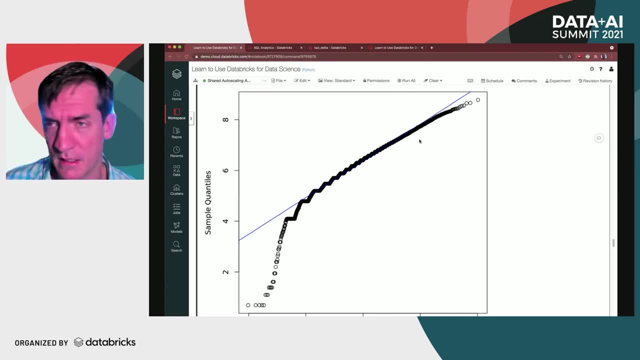 So that I think maybe explains why this is actually in the main log normal but it doesn't quite fit at the low end tier These jumps to the left. I think these are again explained by the quantization I referred to earlier. These are a lot of taxi. trips are rounded. 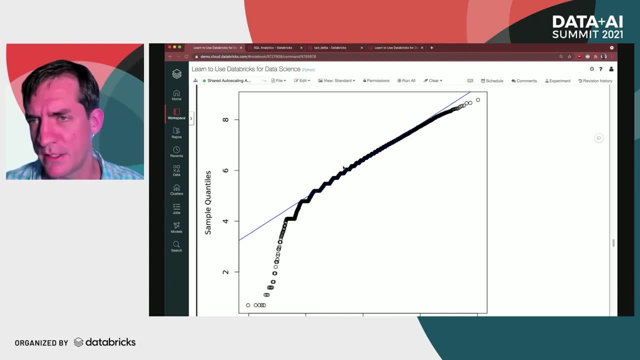 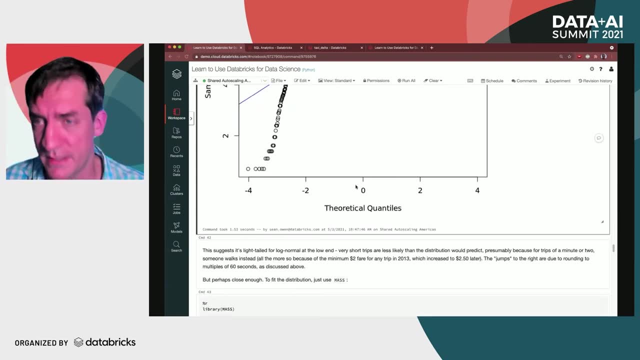 to the nearest 60 seconds, And so I think that explains these kind of odd discontinuities here. But the fit's pretty okay. Maybe I'm interested in the fit because maybe I wanna model the distribution of taxi ride times And I can do that with a lot of libraries. 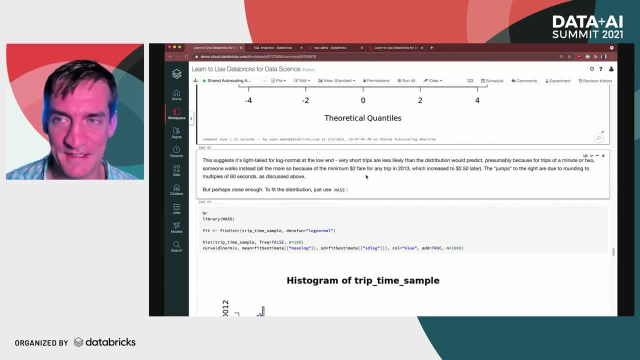 I can definitely do it in R. I know how to do it in R. I don't know how to do it in Python, So let's just use R to do it. So I'm gonna load mass here. This is pre-installed and I'm gonna fit. 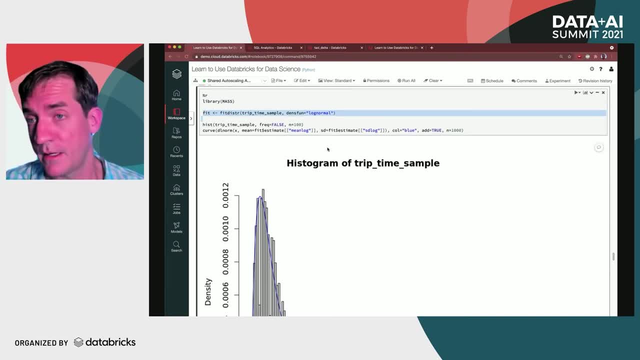 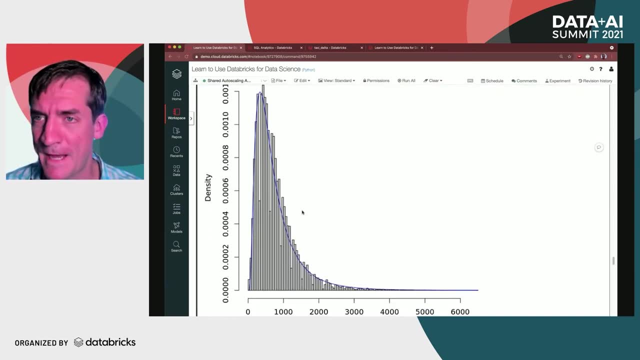 a log normal distribution to it And then just plot my dataset and by frequency with the distribution fit over it And that looks pretty good. I don't know. It seems like a reasonably good fit. There are these weird discontinuities in the histogram. 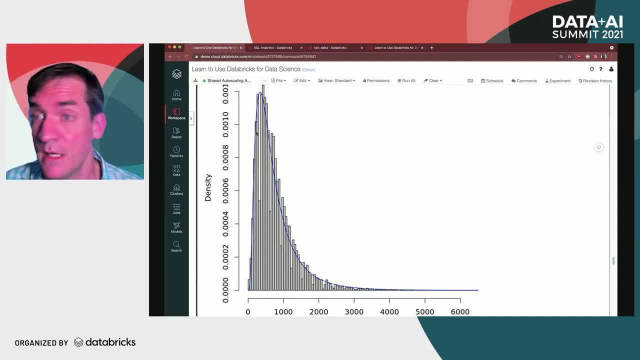 as we've discussed earlier, but this is a pretty reasonable fit. So this is the kind of analysis you need to perform, and you know how to use R to do it. no problem, You can just use the familiar tools in R, And Spark is just here to help you load. 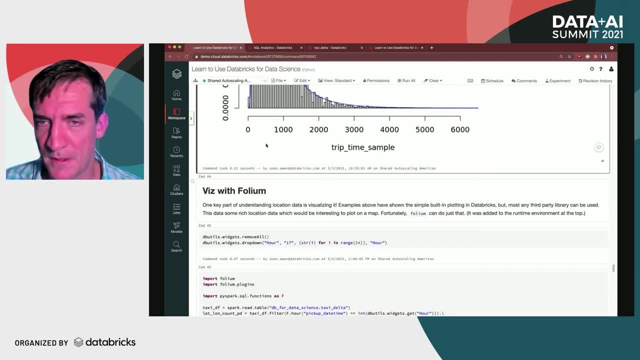 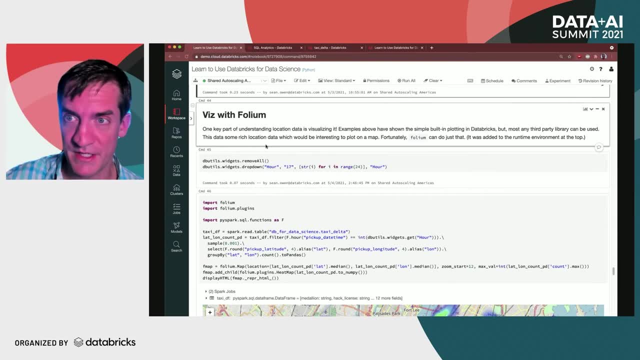 and manipulate the data. Okay, so there's one piece of this data I have not talked about yet, which is the location data. So this dataset has pretty rich data about where these trips started and ended, And what do you wanna do with that? 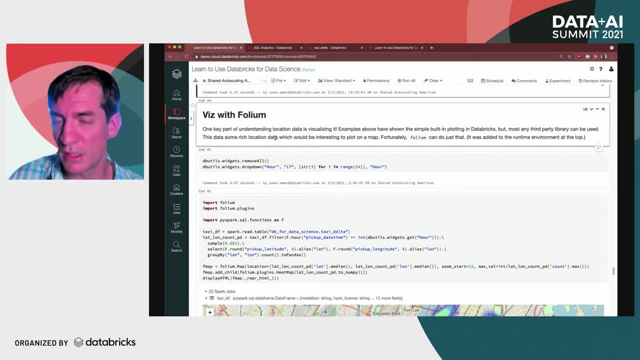 Well, rather than analyze them statistically, maybe we just wanna look at them. We wanna see where trips started and ended on a map. Now, a tool like Databricks does not have built-in tools for plotting location data as a heat map on a map. 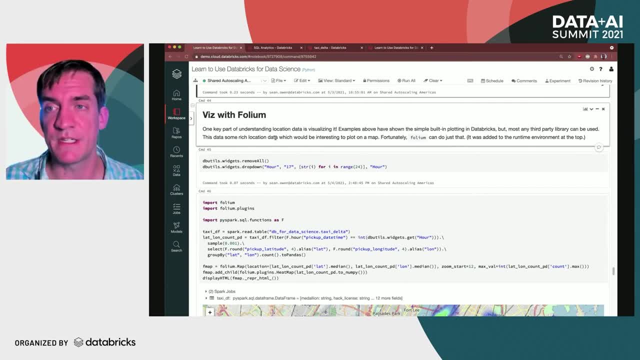 but that's fine because the larger open source ecosystem out there does And the library that can do that easily. one of them is called Folium, And that's one of the libraries I installed earlier into our runtime because I wanna use it here. 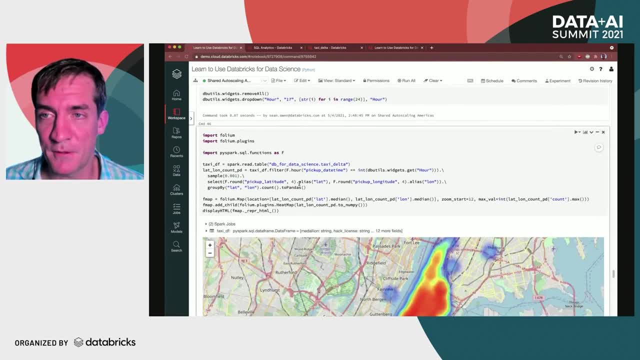 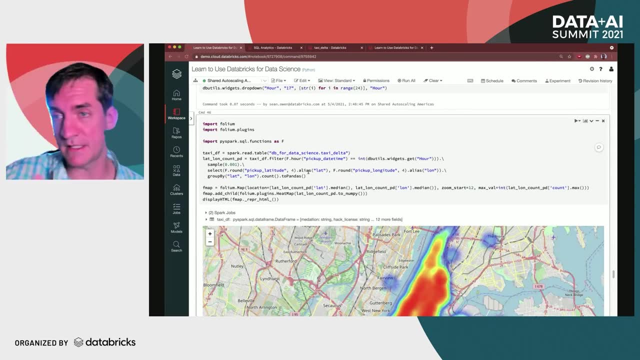 So Folium can do a lot of things, And one of the cool things it can do is plot location data as a heat map over actual maps of the world from Google Maps And because I can easily install it. it because it can accept data and say pandas format and because i can easily grab a sample. 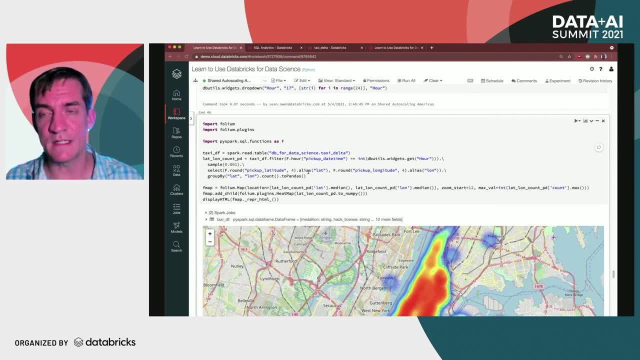 of data as a pandas data frame. these things are easy to put together here in databricks. so here i'm going to read some of this location data. i'm just going to pick up a sample because, again, i don't need the whole data sets and it is. it's too large anyway to pull down, but i don't. 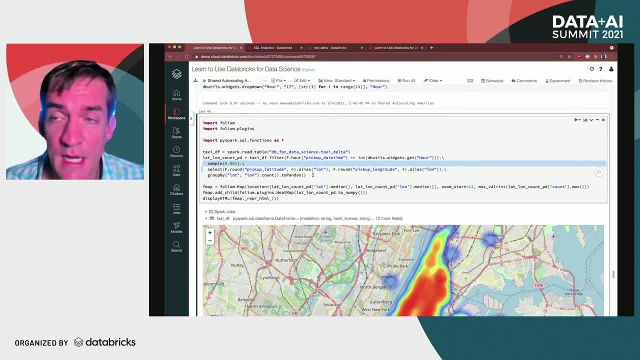 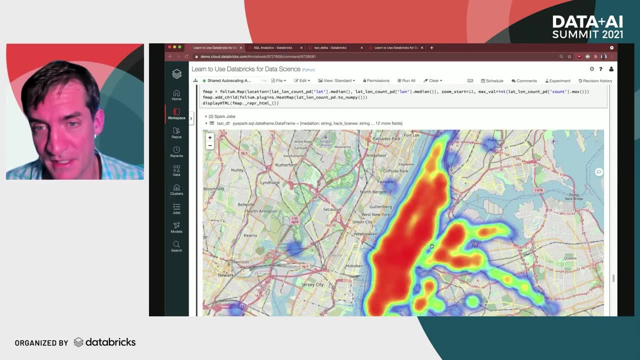 need that to get a sense of where the pickups and drop-offs are, and then i'm going to use boolean to render a plot. it shows me where the pickups and drop-offs are and it's pretty cool. i can zoom in. it's interactive. i can take a look at where people are. this is: these are pickups by: 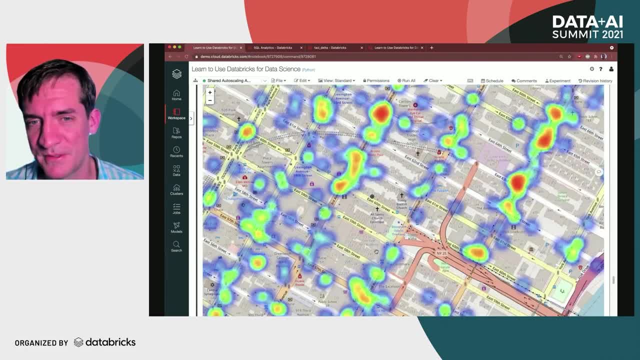 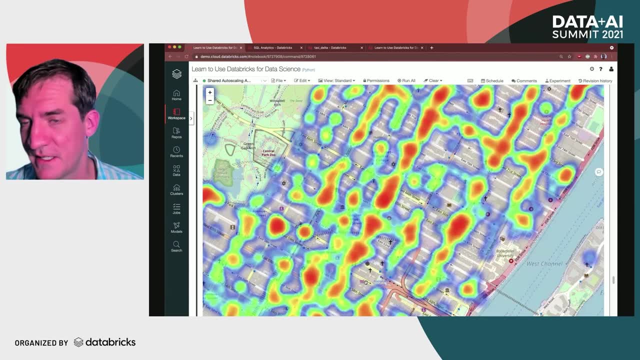 the way, and so obviously it makes sense that people tend to get picked up on corners of intersections, more on avenues and less on these small cross streets. so that's pretty interesting and maybe i want to share this more widely with the organization. but i really don't want to share this entire notebook. we've done a lot of work here. there's 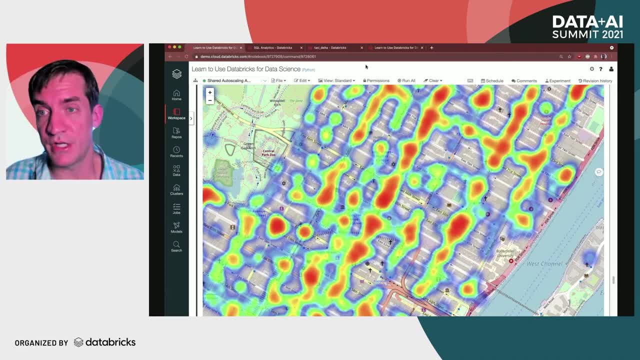 a lot of complexity here and maybe i want to just share this output with someone so they can export themselves. so you can do that too. in databricks, you can export the output of one or more cells as a dashboard, and i've done that here, so let me pop this out here, uh, here, and i can. 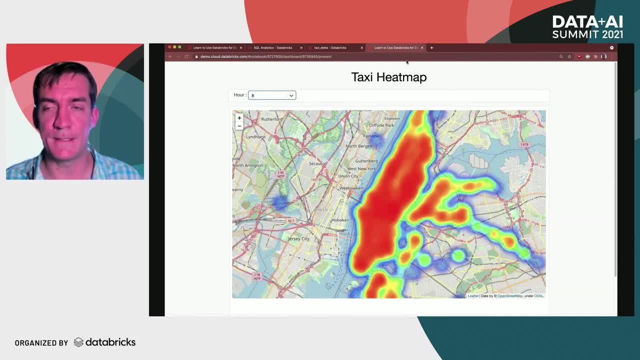 share just this. i can basically share just the output of one cell and actually i didn't comment on this, but i instrumented this cell with a widget that takes that takes as input the hour of the day that we're interested in, so maybe i want to look at what the distribution of pickups. 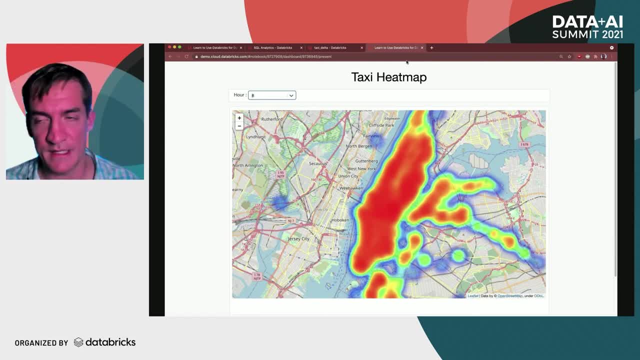 looks like at 8 am versus maybe later at night, and so i can do that, and i can if i instrument it with a widget like this, as the widget changes values, the cell re-executes, the plot re-renders, and so you could share this as a lightly interactive tool with other users, maybe other data. 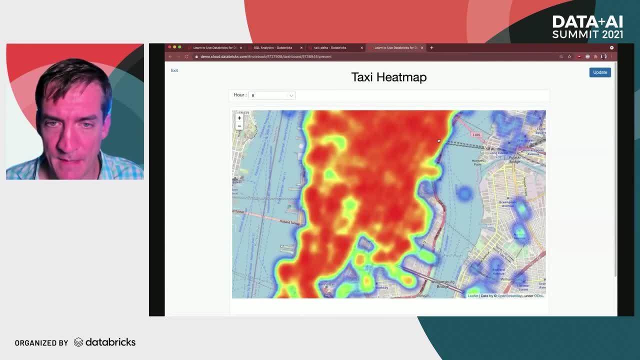 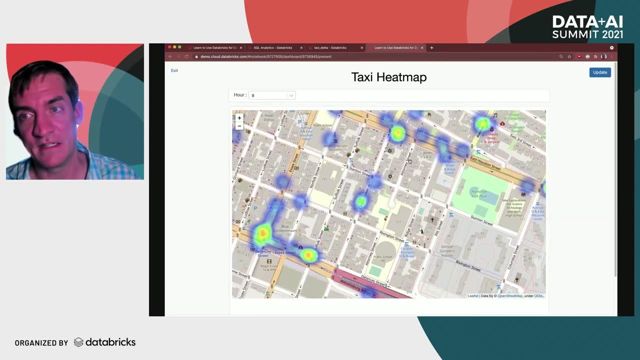 export. so 8 am, let's see what's going on. um, i used to live a long time ago down here on the lower east side and there's not a lot going on. there's not a lot of people taking taxis from from the lower east side at 8 am on any given morning. but if i flip, to my goodness maybe. 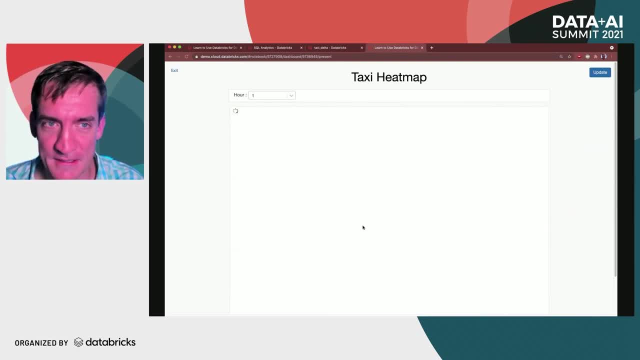 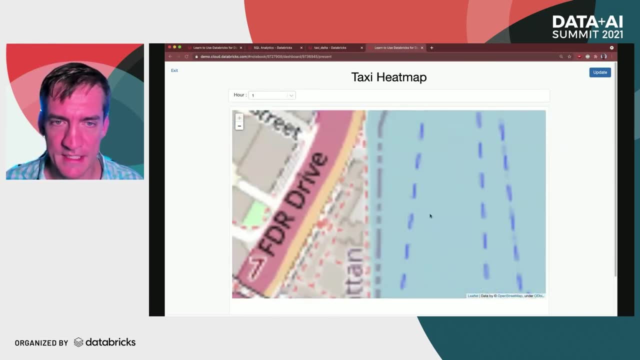 1 am. uh, maybe the picture changes. let's take a look. so i've changed to one. we're going to rerun this whole query, we're going to regenerate the plot and now i can zoom in again and let's see. let's see what's going on on the lower east side. 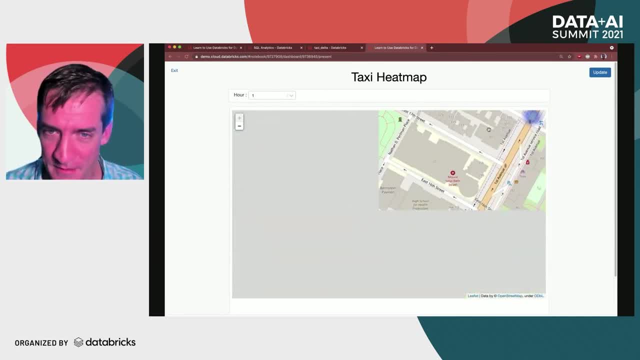 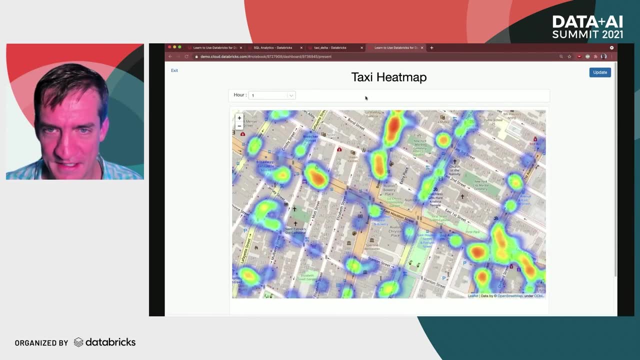 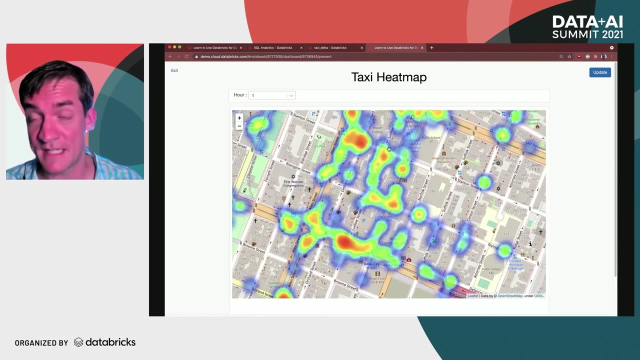 1 am in general. um, i suspect it's a little bit busier. zoom over here. you can already see there's a little more activity. but yeah, dude, i mean, i think anyone that may be familiar with this area would agree that it's more likely that people are taking taxis from this area at 1 am. 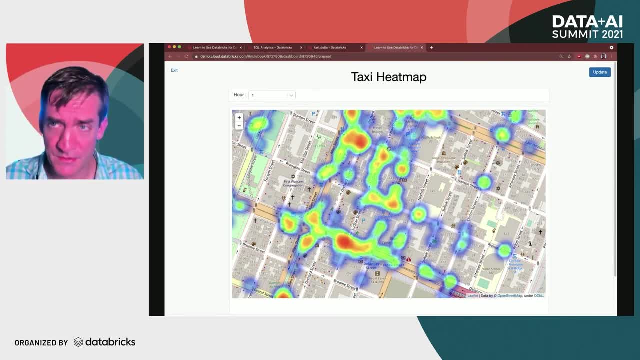 than 8 am, so maybe that's interesting. um, so with a little bit of data science, uh, use of nice open source libraries like folium, you can produce some pretty interesting inter, even interactive, visual visualizations and applications here in databricks which could be useful to the organization. 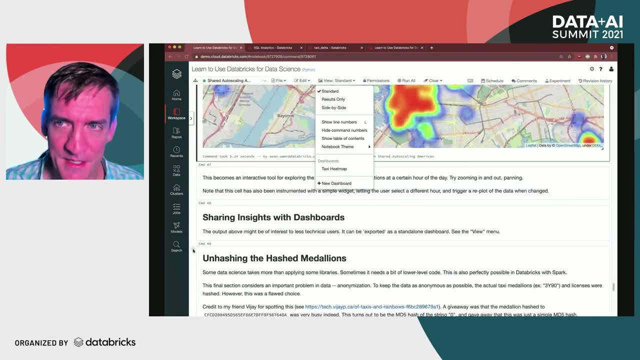 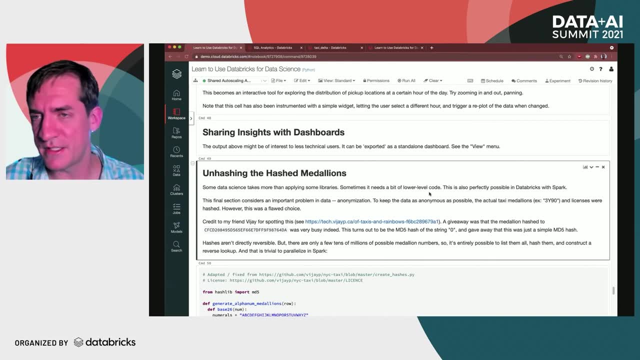 the last thing i'm going to show you as a bonus round, let's talk about those hashed medallions. so sometimes data science is not just a matter of computing aggregations and fitting statistical models. sometimes we have to go a bit off-road, write some code, do something a little more unique. 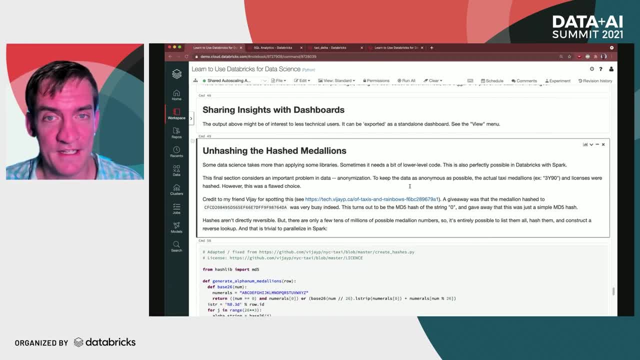 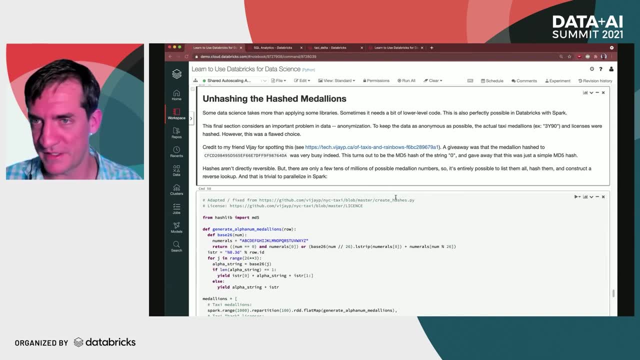 to pursue a particular goal here and i want to show you something interesting, maybe on a different level, but i want to show you something that i've been really fortunate about, this data set that a friend of mine noticed, uh over 10 years ago, uh, eight years ago, about this data set- his name. 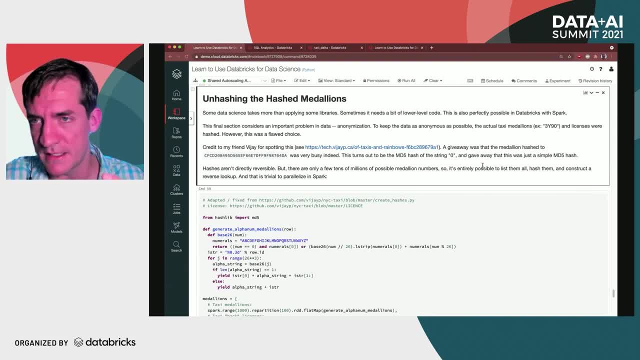 is vj and he looked at this data set and noticed that, yes, these medallions and these hack license hack license numbers were hashed. they were hashed in order to protect privacy. they didn't want to publish the actual medallion number involved in each transaction, so they hashed them and that's a. 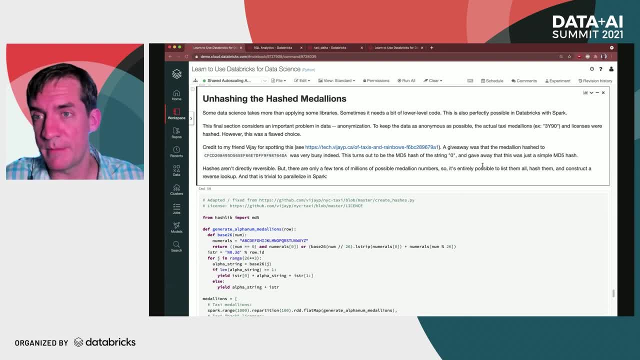 good idea. i mean, hashes are generally not reversible, but if you look at the hash values, you can see that there was a medallion id that had almost 22 000 rides in a year in new york, without revealing what the medallion was. however, there 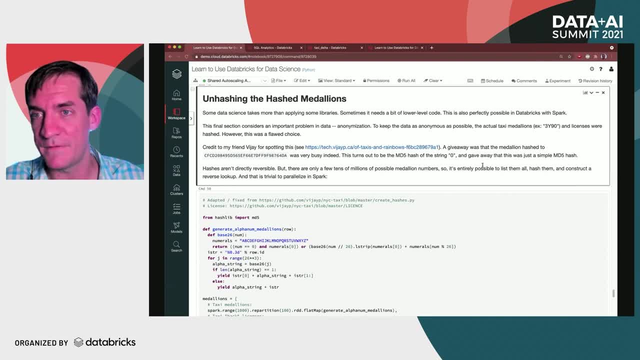 was a problem, um. so he noticed that if you looked at the hash values, you saw some kind of strangely familiar values here, and he quickly figured out that what they must have done is simply apply, uh, an md5 hash to the strings, to the, to these um medallion and 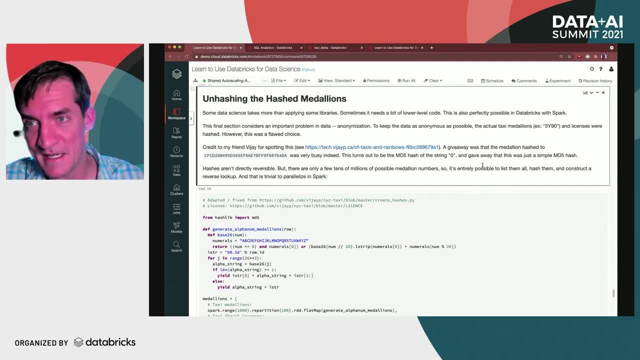 hack license strings. now, that's not a terrible idea, but it was pretty obvious and he figured this out because- um, not because- they hashed the, the empty string, and i think some developers out there will recognize the hash of the empty string- md5 hash- but a lot of the values turned out to be. 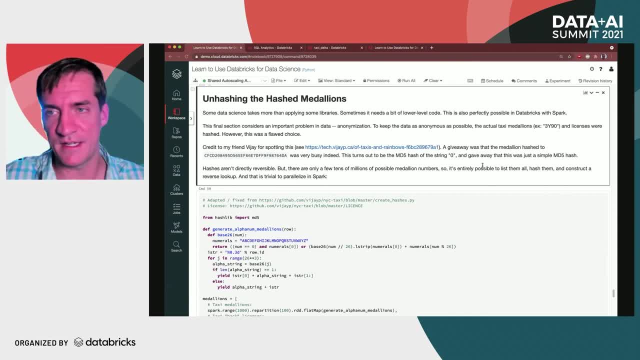 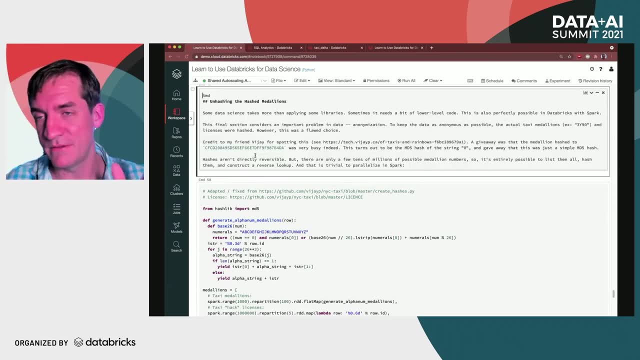 zero and the hash of the string zero is this, uh, this that you see here, and this was the giveaway about what they'd done. now, that's still fine, because the hash is not directly reversible. however, there are only so many possible medallion ids and hack license ids. if you've been in new york, you know. 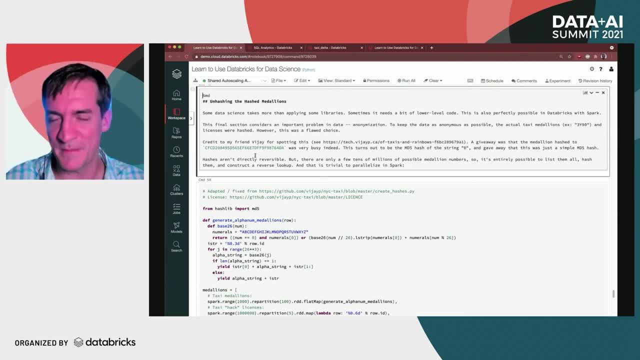 that the medallions look like three y, nine zero. there's only so many of them, they follow a particular format, so it's entirely possible to generate all of them, hash all of them and then revert, generate a reverse lookup table. now that could be computationally, um, sound computationally. 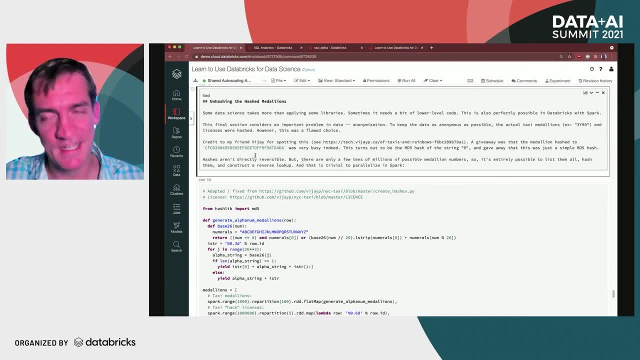 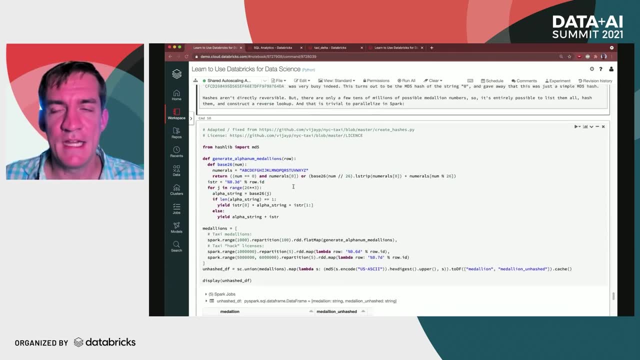 difficult, but it's not because there's only about 20 million possibilities and this you could do on your own, but just for fun i ported this to spark and here in this bit of code, and i've had to write some more lower level python code to do this. 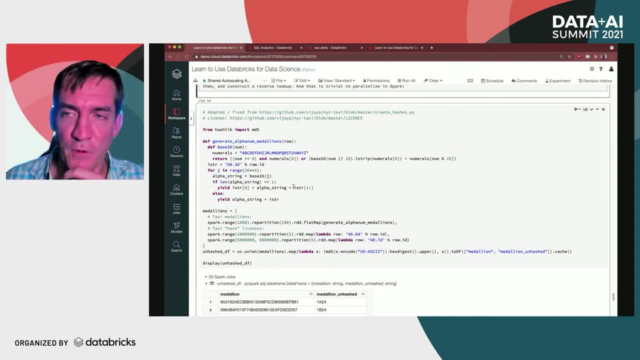 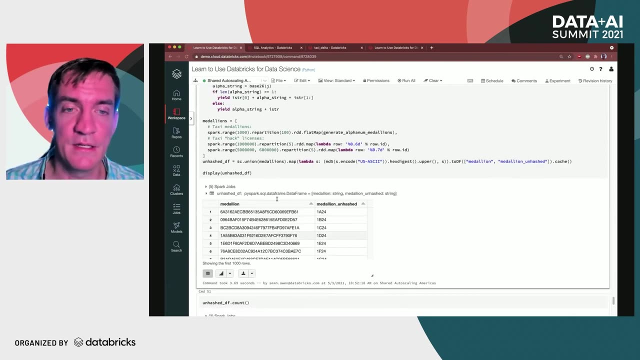 but i can do this in spark because spark's available. in just about four seconds, i generated all the possible unhashings of all possible medallions and hack licenses in new york city, like. so, given that, of course, that's a data set that i can join on the original hash data to tell. 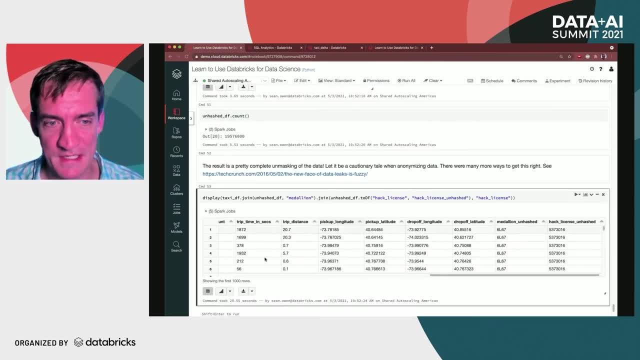 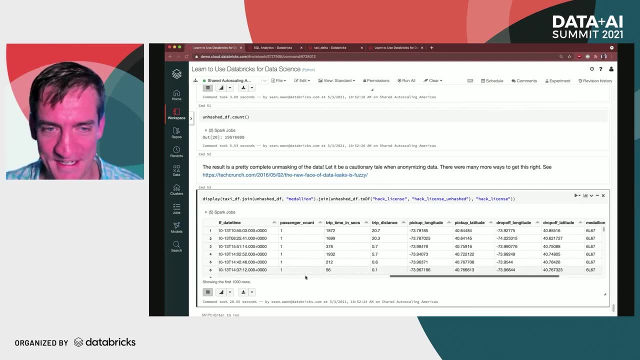 me what the actual medallion will look like in your home, so i'm going to go ahead and show you. that is for each of these rows. So I've done that here, you know, generated about 20 million possibilities, joined it here and yeah voila, Even though we start with hashed hack licenses. 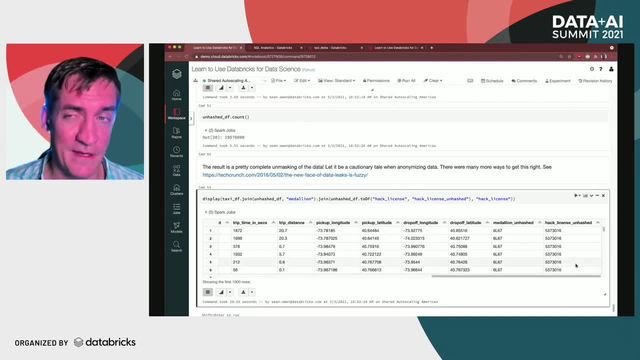 and medallions, we can easily uncover the original value. Now, I'm not suggesting you should do this, I'm not suggesting this is the goal of data science, but if you need to do something like this, it's nice to have the tooling available here. I can write lower-level Python code and 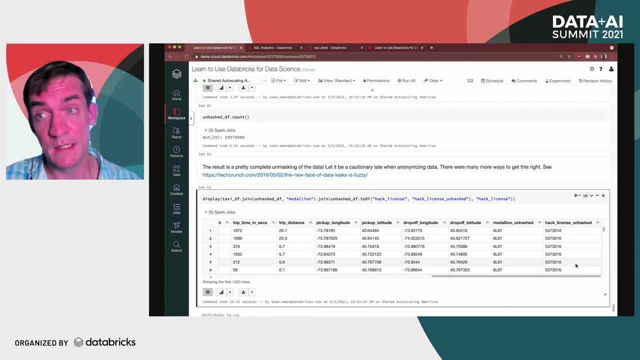 distribute it if I need to throw a lot of compute at a problem like this. It's also a cautionary tale. If you are hashing data to release it to the public in your data set, please don't just do this. Please salt your data and then hash it at the very least, Because we have a bit of time. 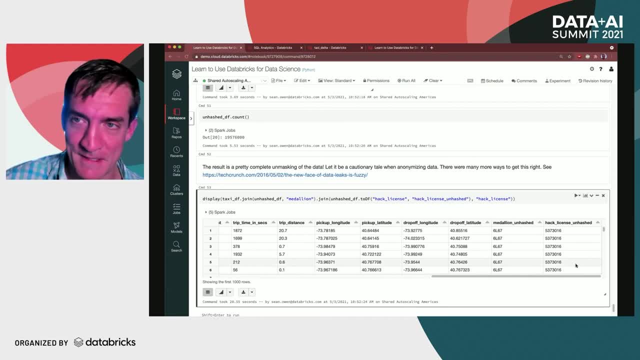 I'll tell you as a coda here: unfortunately, people picked up on this and found photos of celebrities that were maybe getting out of a taxi at certain locations at a certain time and used this data set to go work backwards and figure out how to do this. So I'm not suggesting you should do this. I'm not suggesting you should do this. 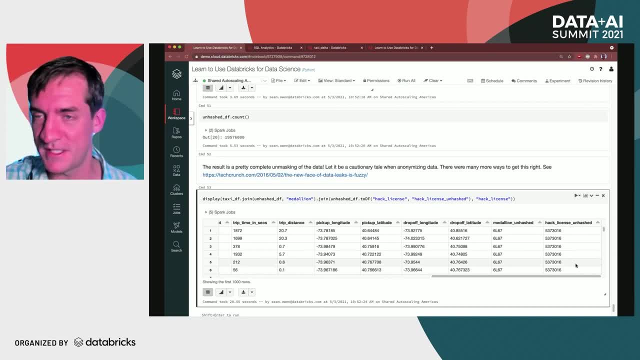 So I'm not suggesting you should do this. I'm not suggesting you should do this, But what the source of the trip was. because if you know that a person got out of a well-known place at a certain time and you can read the medallion out of the photo, then you can do something like this to 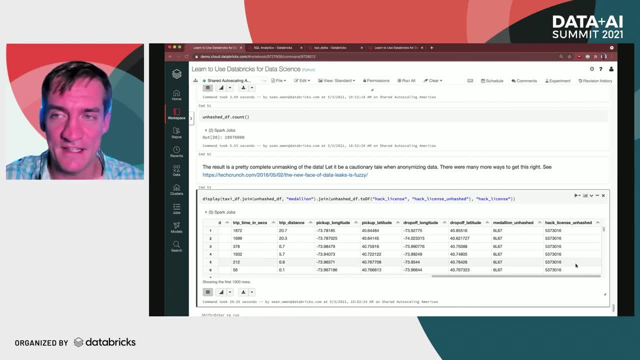 figure out what trip it was and work out where the trip started. And there's actually a different data set here that includes things like tip, So you can work out which celebrities are good tippers or not. And that was unintended, of course, And again, I'm not suggesting this is. 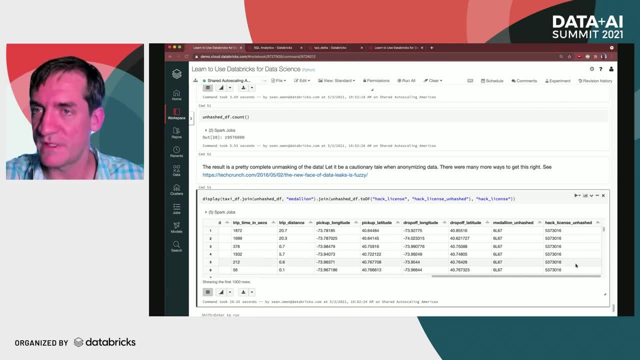 something you should do, But for the resourceful data scientists, it's the kind of thing you'd absolutely can do or should be careful about not allowing in your own analysis With that. thank you very much. I hope this has been a useful overview of what Databricks looks.